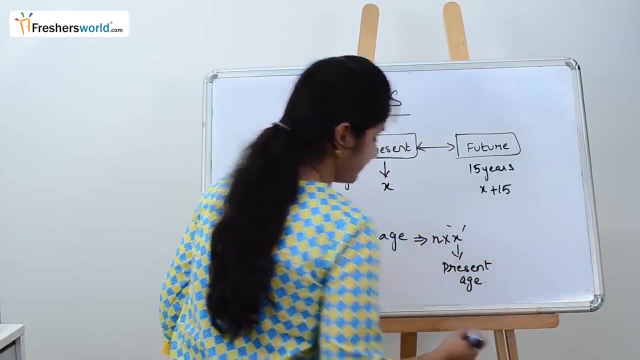 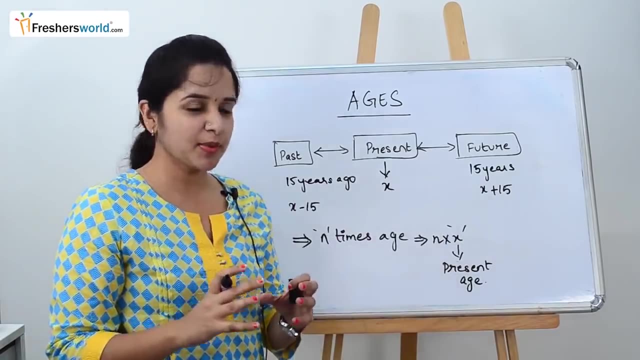 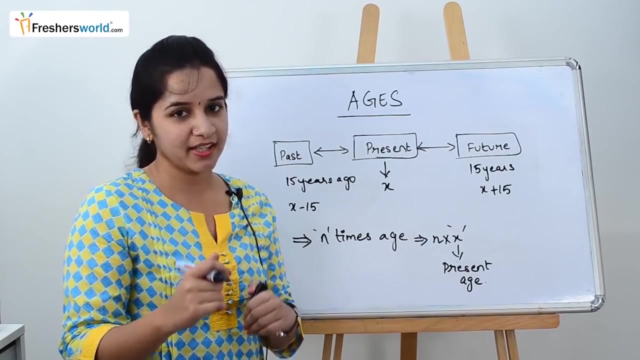 would have given so to solve any ages problem. these four concepts should be very clear. so ages problem is not about how you gonna solve this. it's about how well you understand the sum, how well you are segregating the sum inorder to get the answer. better to understand the. 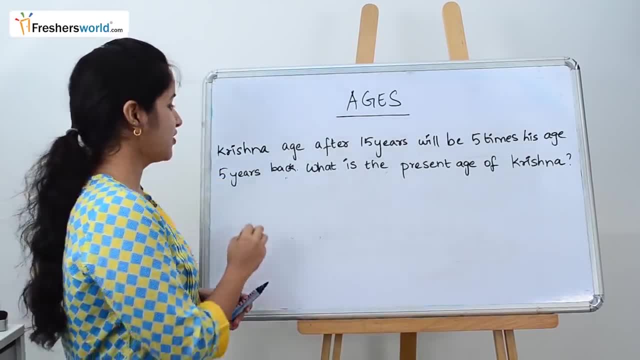 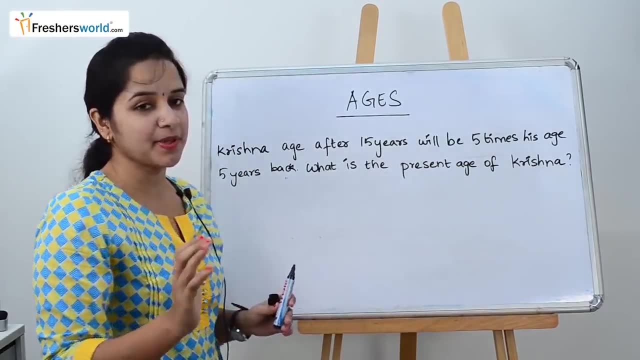 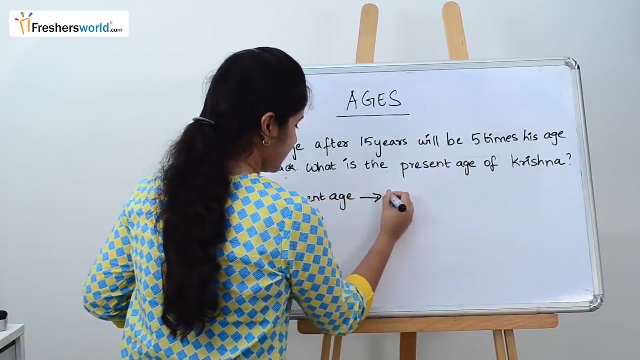 ages concept better. let's solve a couple of problems. so the given question is: Krishna age after 15 years will be five times his age, five years back. so what is his present age of Krishna? So we know that we are going to take the present age as x. So what are? they Read the question again: Krishna's age after 15 years. So the future age of Krishna x plus 15 will be 5 times his age 5 years back. So old age is x minus 5.. So let's. 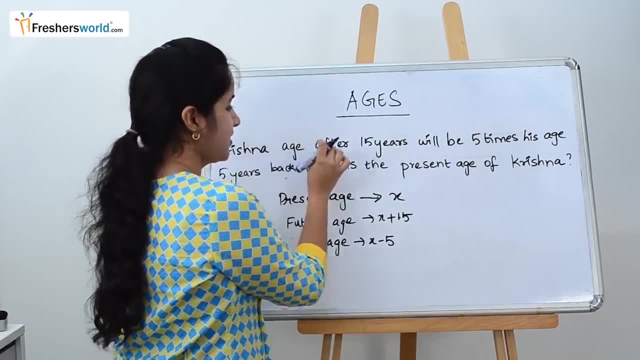 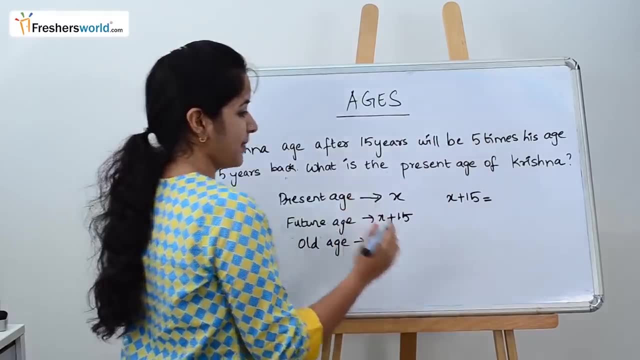 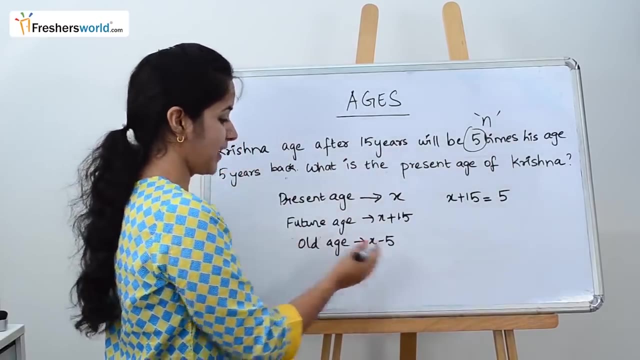 now create an equation. Read the question again: Krishna age after 15 years x plus 15 will be 5 times his age 5 years back, So 5 times. here is remember that n times, So 5 times his age 5 years back, So x minus 5.. So let's just solve this equation: x plus. 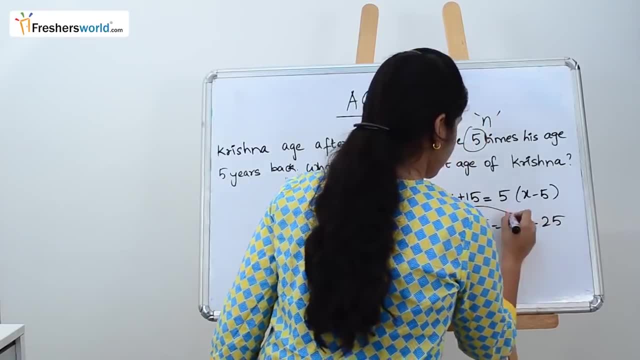 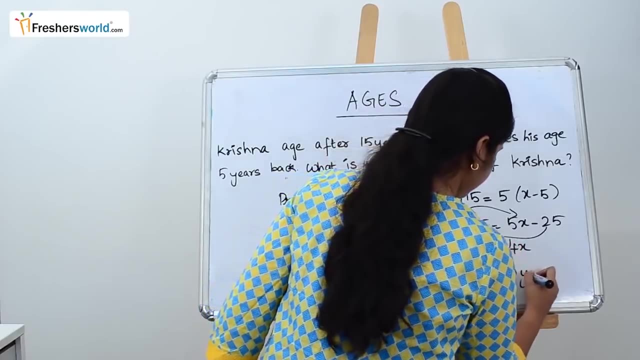 15 is equal to 5x minus 25.. So let's take x here, So it is 4x, and we are taking 25.. 25 here, which is 40. So x is equal to 10.. So the present age of Krishna is 10 years. 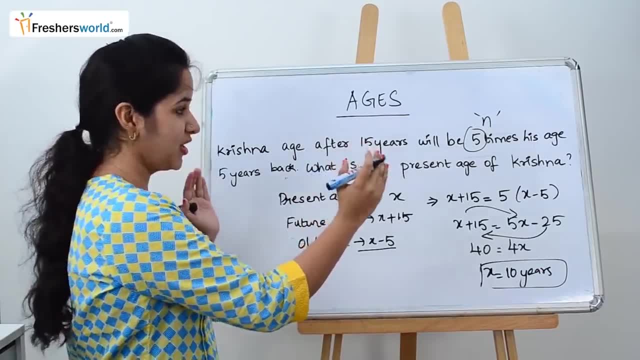 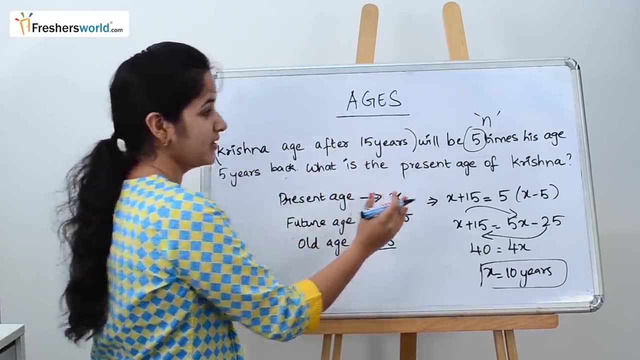 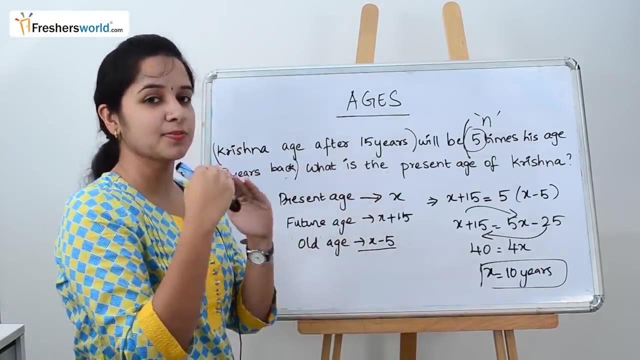 So in this example. so once you segregate the question into 3, you will be able to answer the question. Let's take the Krishna age after 15 years, Take it as a separate factor and will be 5 times his age, 5 years back. So if you segregate into the present age. 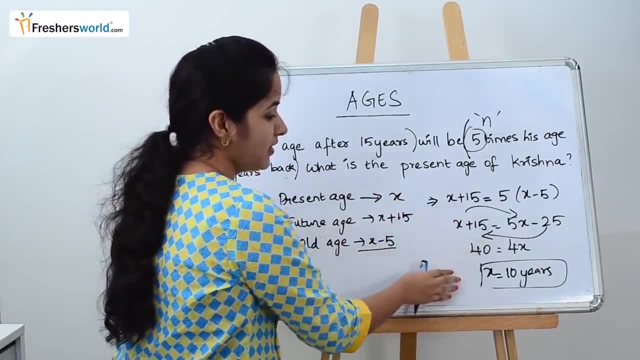 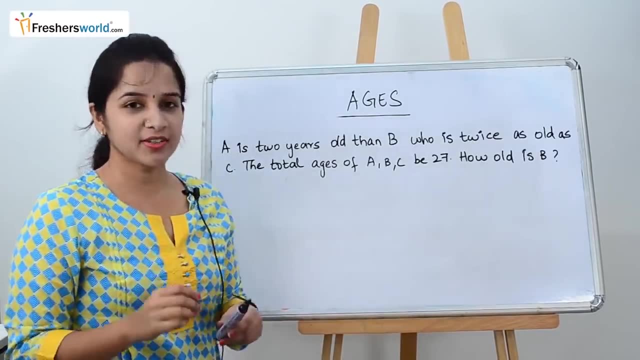 past age and the future age. it will be easy for you to find The equation. once you know the equation, it will always be easy to find the x. Let's solve another question. So the next question is: A is 2 years older than B, who is twice as. 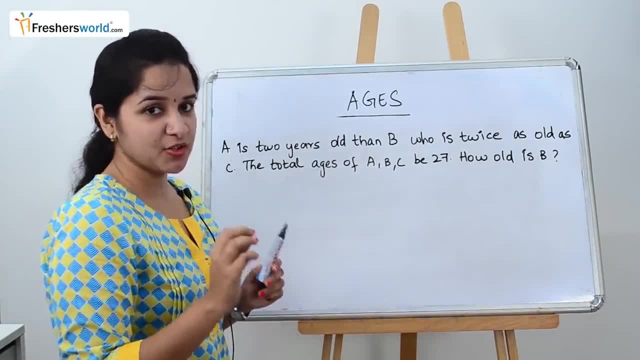 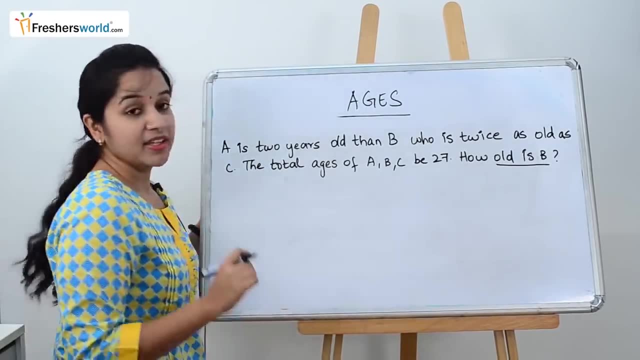 old as C. So they have given the total age of A, B. C is 27 and they are asking us to find how old is B. So we always have to find which is the x variable here. Okay, they have. 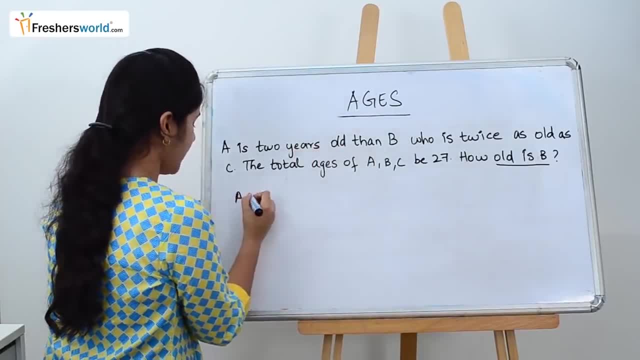 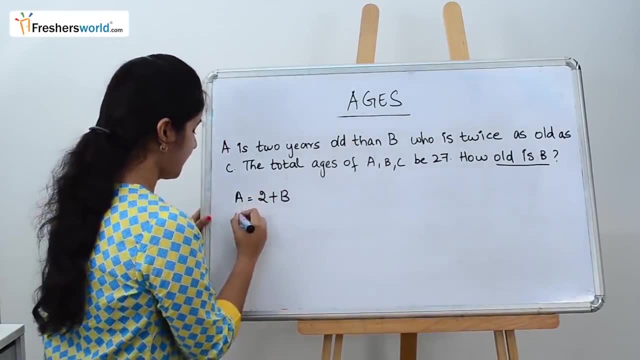 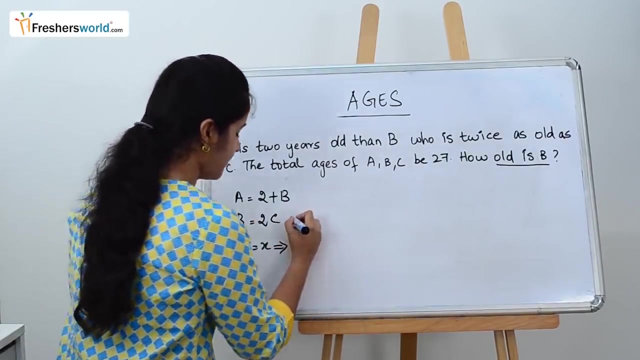 given: A is 2 years older than B, So A is 2 years older than B. So B is twice as old as V. So we can take C as X. So if you know C is X, then your B becomes 2X and your A becomes 2 plus B, which is nothing but 2X. 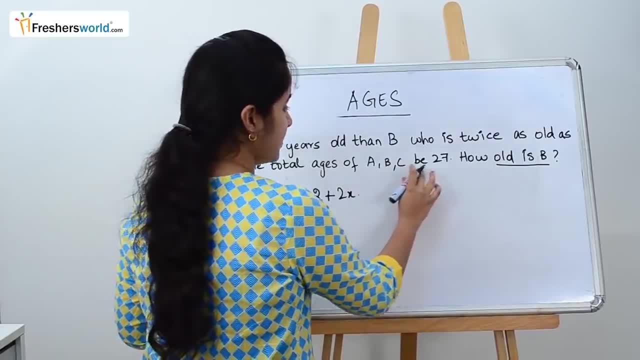 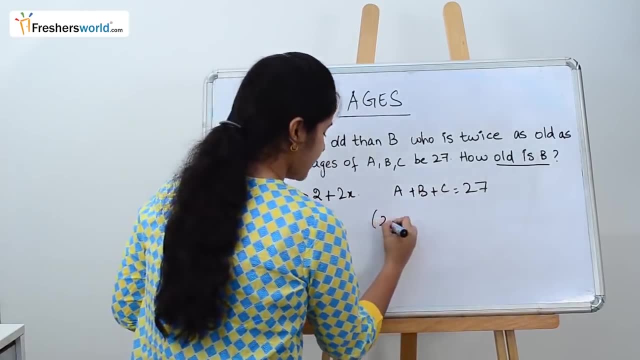 So what are the other things they have? given Total number of ages is 27.. So A plus B plus C is equal to 27.. So what is A, 2 plus 2X Plus what is B, 2X plus X, 27.. 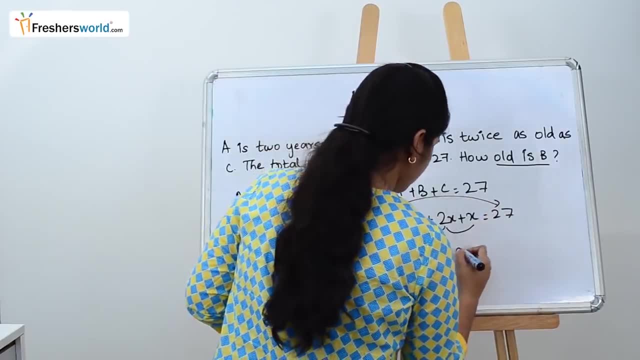 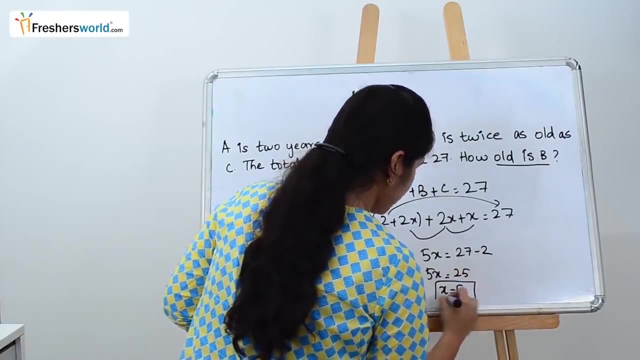 So 5X, we take 2 here, So 27 minus 2, 5X is equal to 25, X is equal to 5.. So we found out: X is equal to 5.. But is that the question they have asked? No, 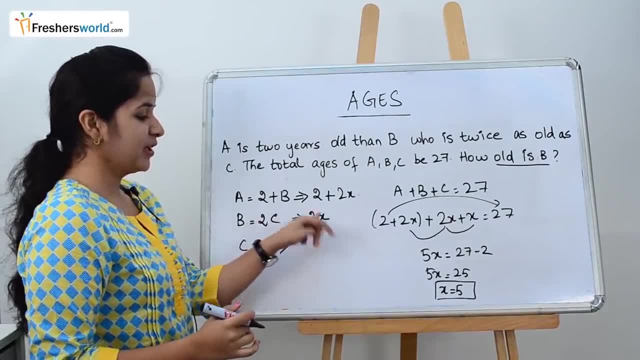 They are asking: how old is B? So what is B? B is nothing but 2X. So B is equal to 2X, So 2 into 5.. So 2 into 5 is equal to 10 years. 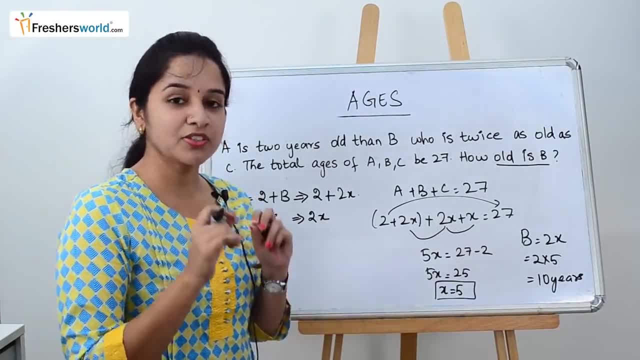 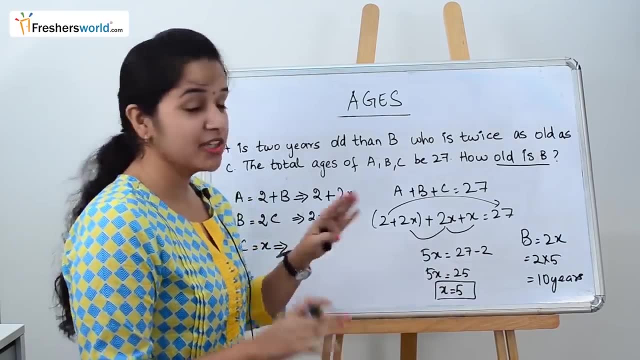 So the common mistake people make it here you will find the X. You will also have the answer as 5 in your question, So you will automatically click 5 and then finish off the question. But read the question again. Are they asking for the X variable? X is nothing but C here. 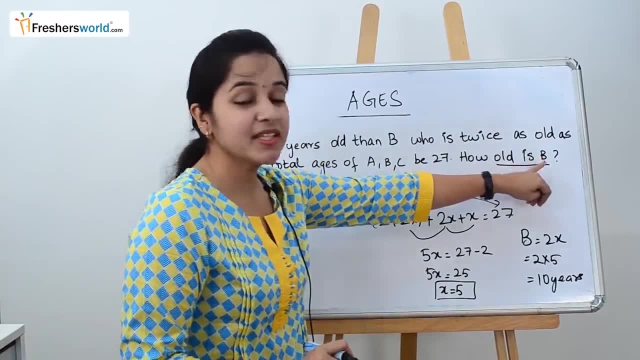 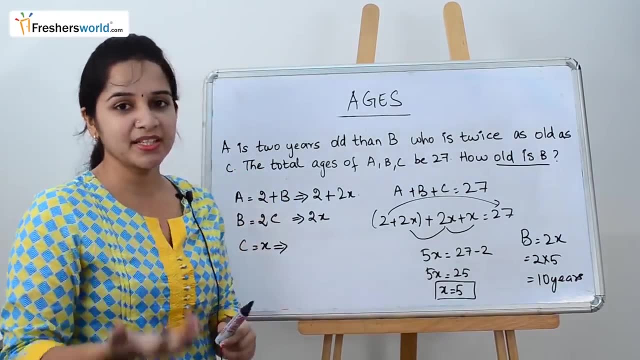 They are not asking for C's age. they are asking for B's age. B is nothing but 2X, and that's why we get to know that it is 10 years. It's not only for this. they may also suddenly ask A and B's age. 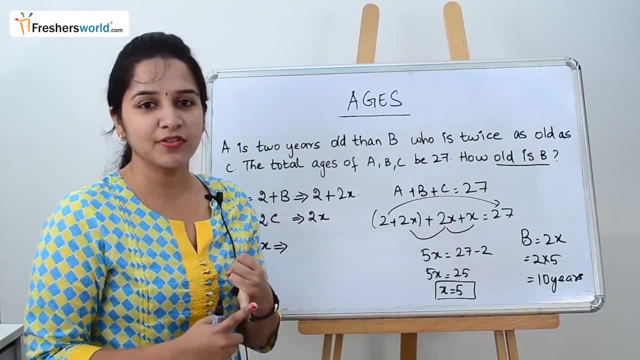 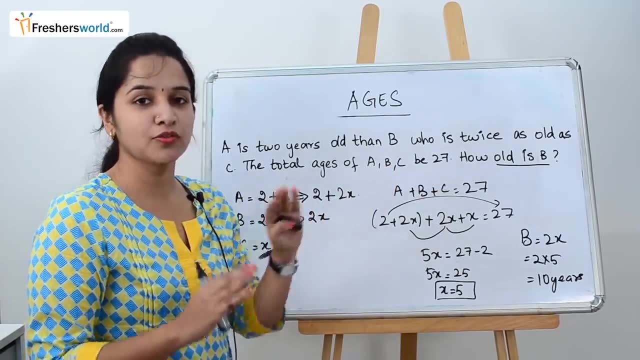 So always make sure that you read the question. The main thing first you have to see in a problem is: what is your X Based on that? segregate it into three different equations, Then you form your question to find X. Let's solve another problem. 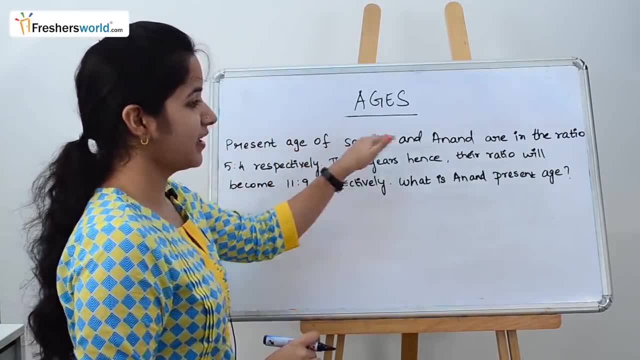 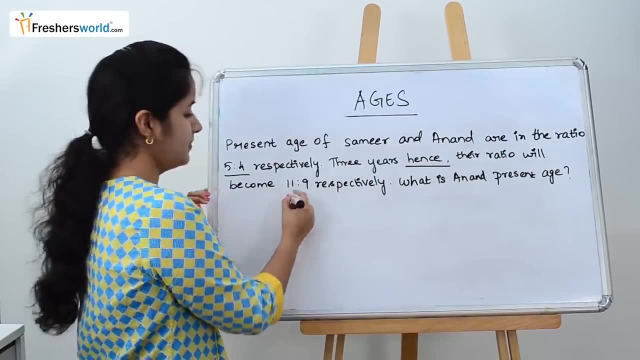 So the next question that they have given is Present age of Sameer and Anand are in the ratio of 5 is to 4, respectively 3 years. hence their ratio will become 11 is to 9.. So what is Anand's present age? 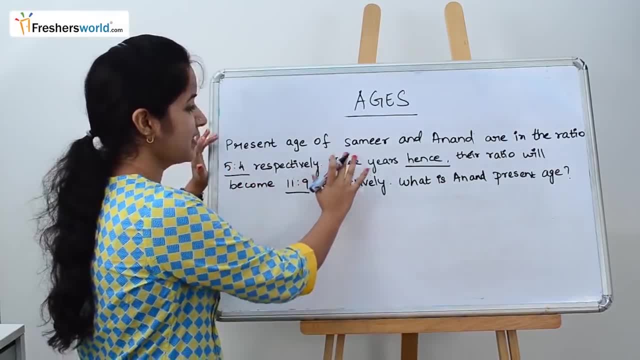 So let's write whatever is given in the first type of sentence. So present age of Sameer and Anand are in the ratio of 5 is to 4 respectively. So present age of Sameer and Anand are in the ratio of 5 is to 4 respectively. 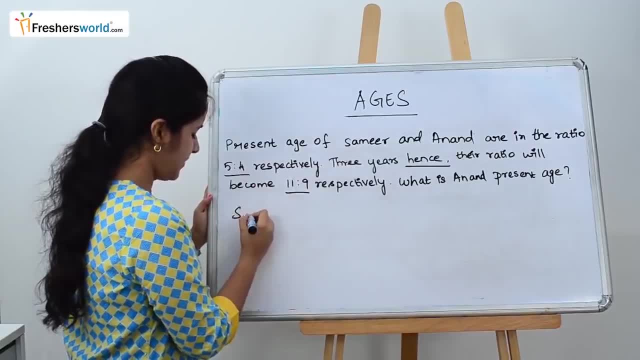 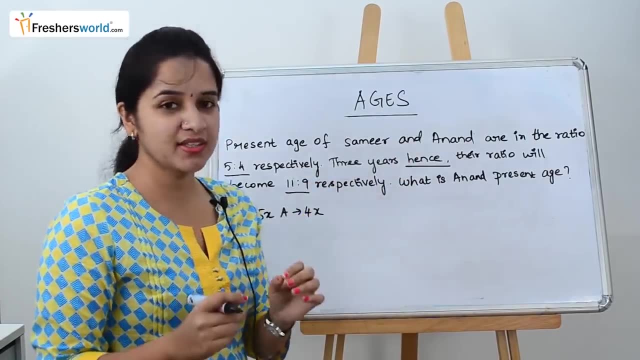 days they have given in the ratio of 5 and 4.. Let's take, for Sameer it is 5x and for Anand it is 4x, What they have given 3 years hence. So hence we know that we have to add. 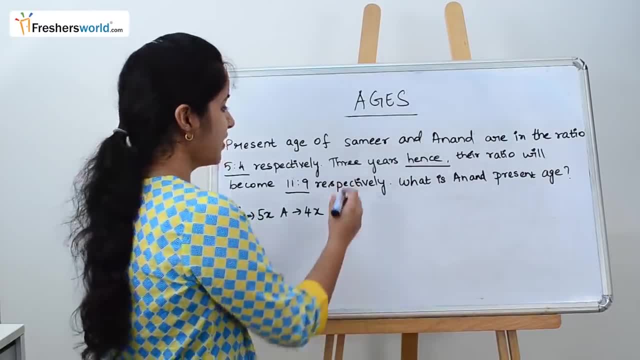 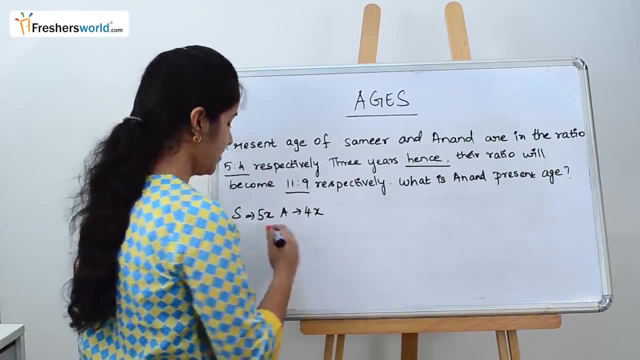 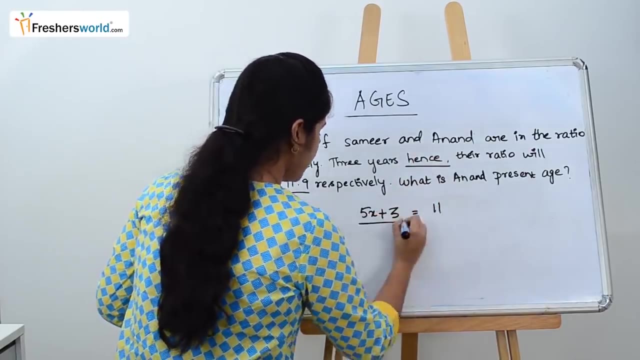 it. Hence why are we adding it? Because it's a future age. So they are telling that after 3 years their ratio will become 11 is to 9.. We know that ratio will always show it in a fraction. So they are saying 5x plus after 3 years will become 11.. Similarly 4x. 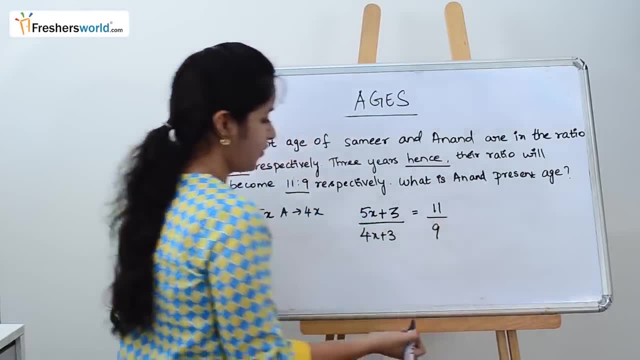 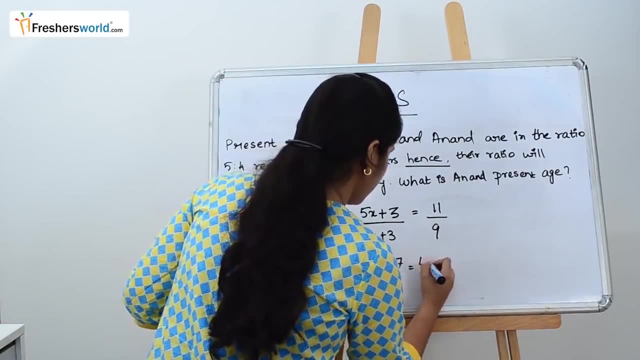 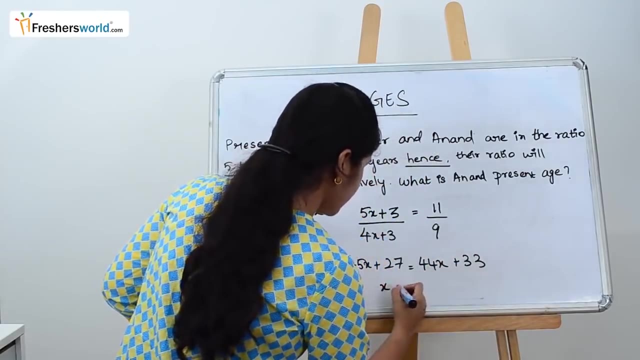 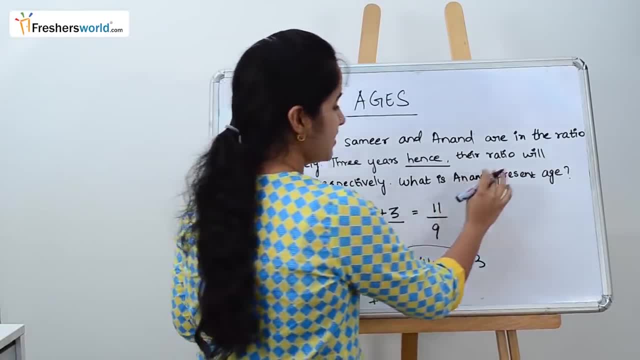 that x is equal to 6.. So what are they asking? What is the Anand's present age? So we know that this is the present age, which is nothing, but for Sameer it is 5x and for Anand it. 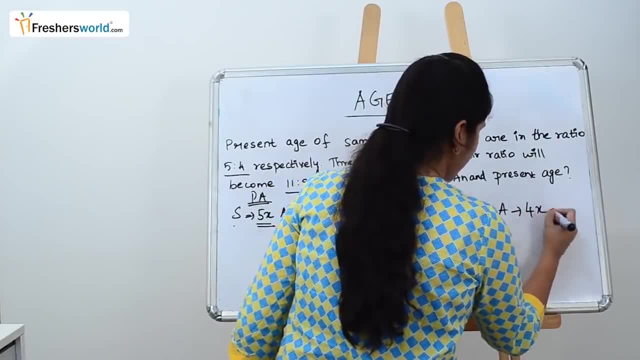 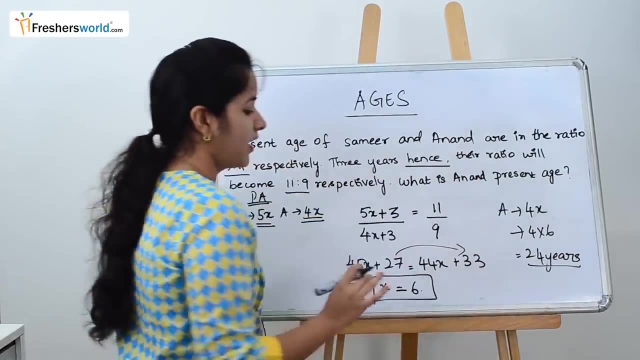 is 4x, So we have to find Anand's age. So 4x is nothing but 4 into 6. So it's 24 years. So now we know Anand's present age. So in this type of problem, if they are going, 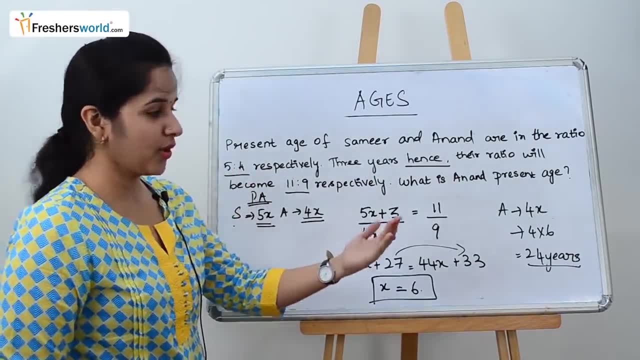 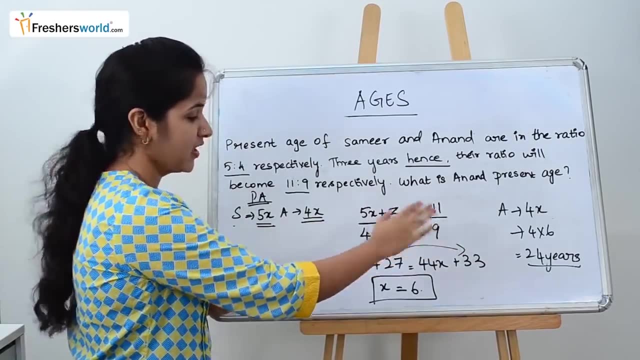 to give it in ratio check. if they have given the future one- or sometimes they would have given 5 years before- Then you have to subtract it here and then equal it to the ratio that they have given. So if you do that you can easily. 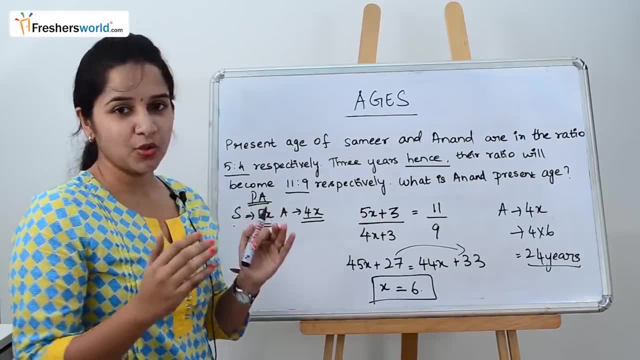 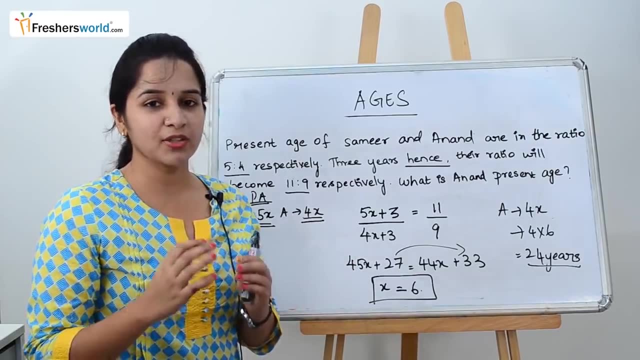 find it x. So, as I say always, always, separate your question into different brackets so that you can understand the question better before solving ages. So there are no tricks or something to solve the ages problem. It's all how you understand the question and how you segregate. 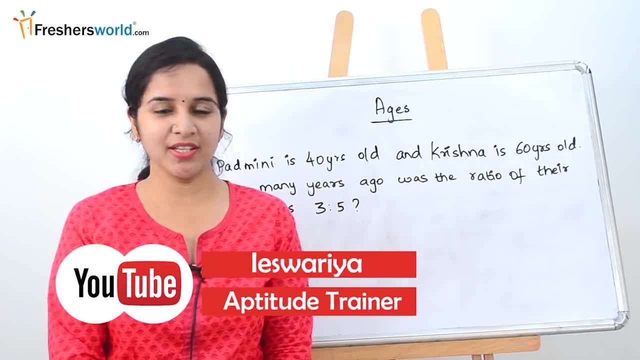 the question in order to find the answer. The topic that we are going to look today is the part 2 of ages, So in the part 2 of ages, we are going to look at the question called the basic concepts of ages. In the part 1 of ages, we discussed about the basic 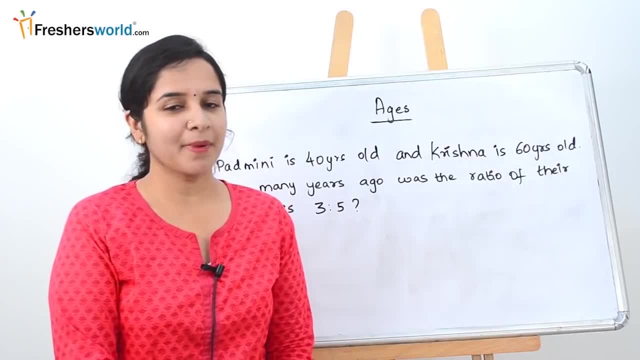 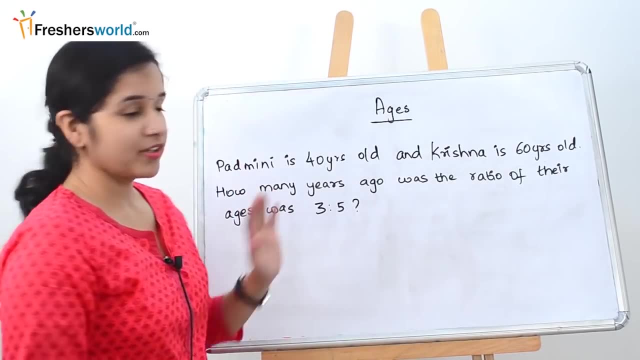 concepts in ages and as well as the simple sum to it. So in the part 2, we will be discussing a much tougher problem compared to it and how easily we can solve it. So the first question is: Padmini is 40 years old and Krishna is 60 years old. How many years ago was the 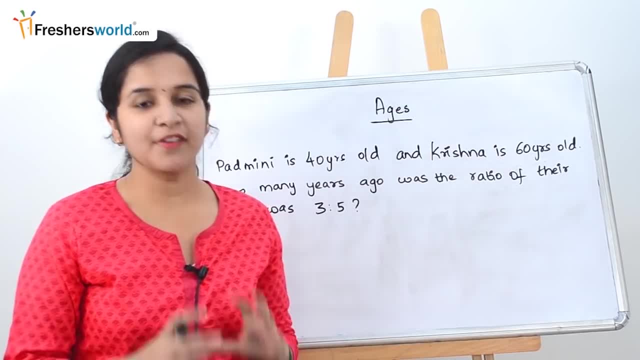 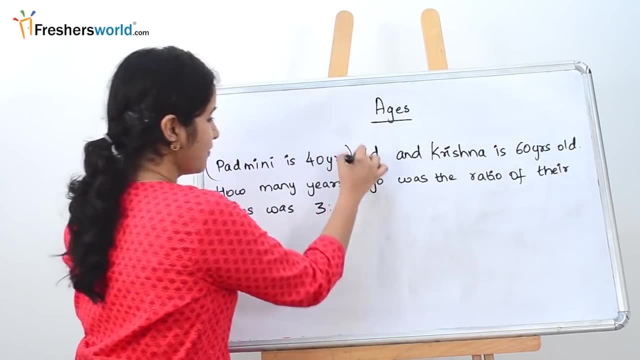 ratio of their ages was 3 to 5?. In the part 1 itself, I have clearly told you you have to segregate the question into brackets such that it is easy for you to find it. So Padmini is 40 years old. 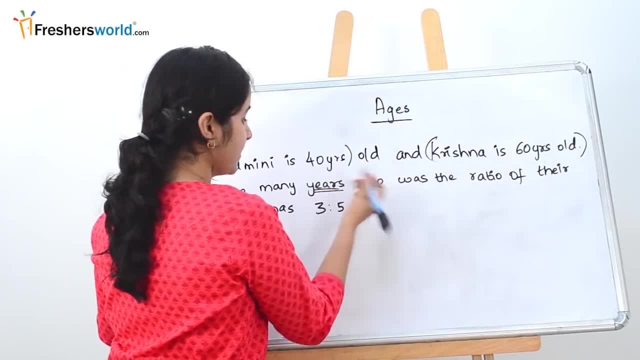 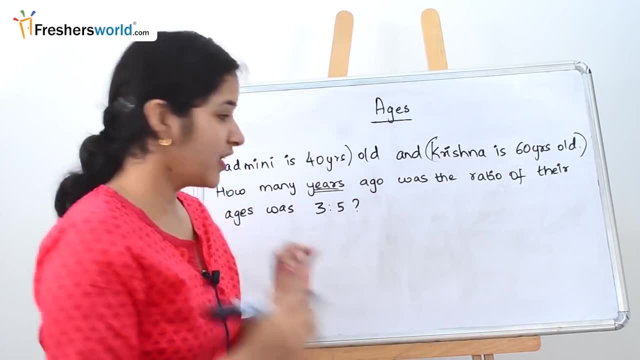 years old, how many years ago? so we have to find number. of years ago was the ratio of their ages was 3 is to 5. so they didn't mention the years ago, but the word ago means that we have to subtract it. so Padmini by Krishna is: 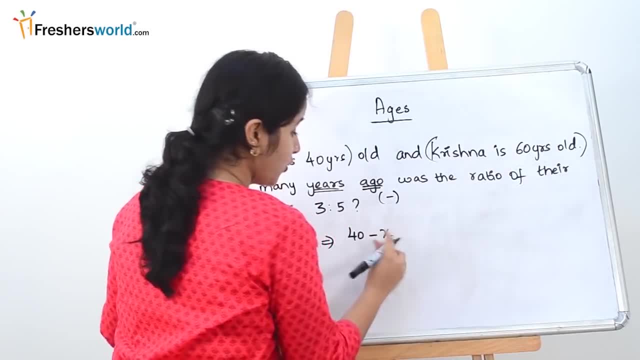 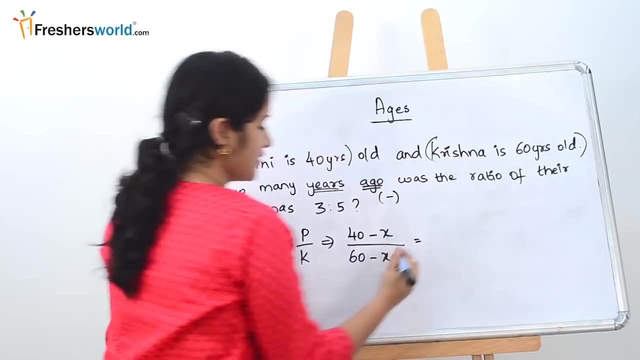 nothing but Padmini as 40 years old, when we don't know how many years ago, divided by Krishna was 60 years old. we don't know the years ago again was their ratio 3 is to 5. it's very simple to solve. once you find this equation, all you have to. 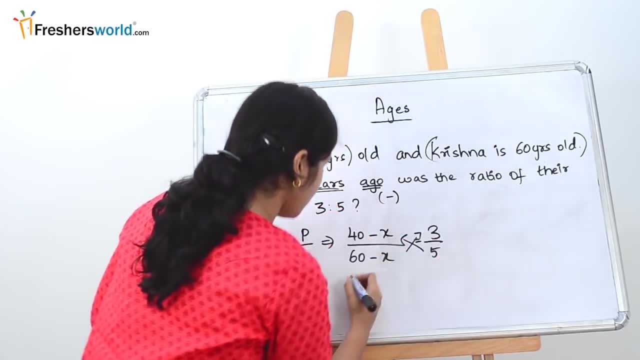 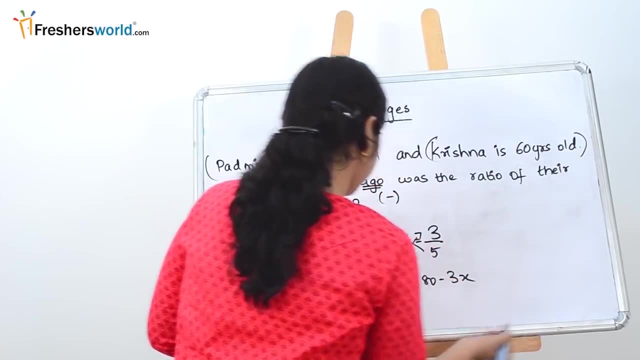 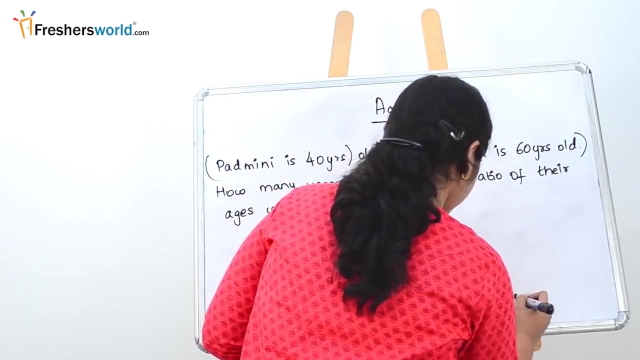 do is find the X just cross multiply. so 200 minus 5x is equal to 180 minus 3x. you just move the 5 there. so 2x is equal to 20 and X is equal to 10 years, so 10. 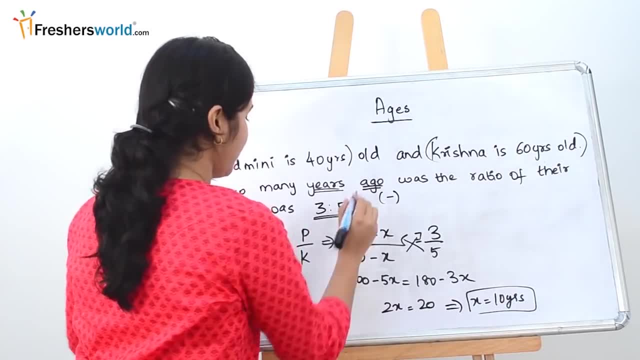 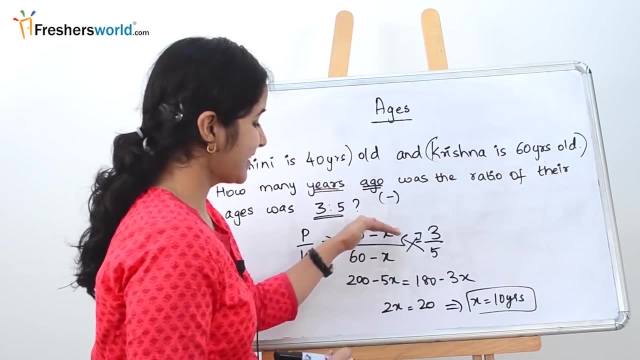 years ago. their ratio of their ages, where it's 3, is to 5. so how did we solve it? so we know their respective ages, we put it in a fraction, wise, and put X as the number of years ago and equate it to the ratio that they have given. if you just 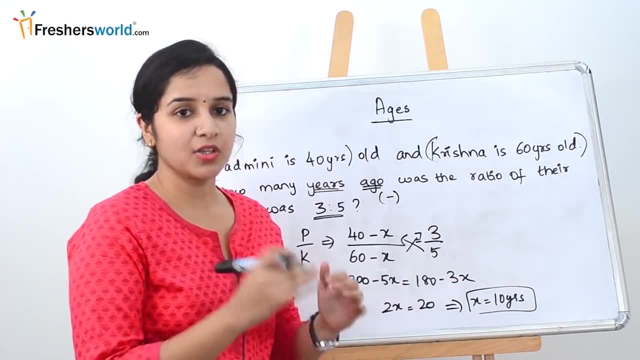 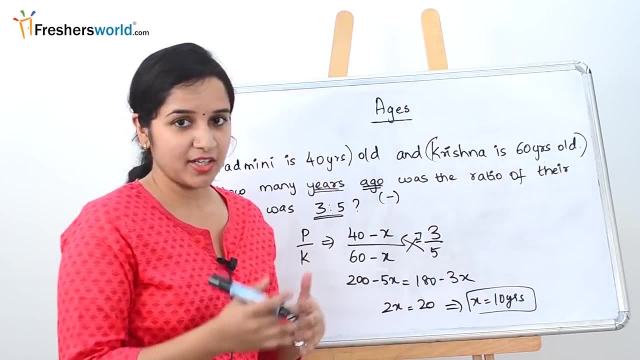 cross, multiply it and find X. you will be able to find the years ago in which the ratio was so and so. similarly, they will just interchange the value of their ages and then give you a various ratio proportion. based on that, all you have to do is follow the same method. only the values will change here. to find the 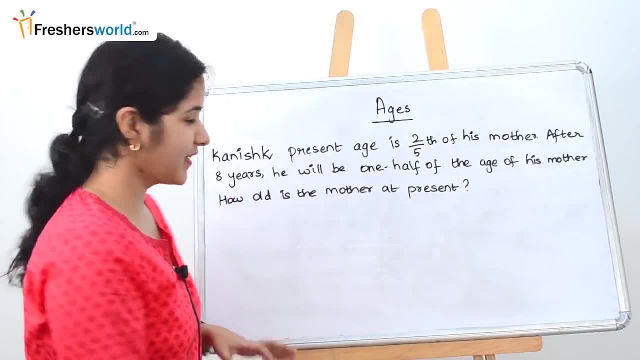 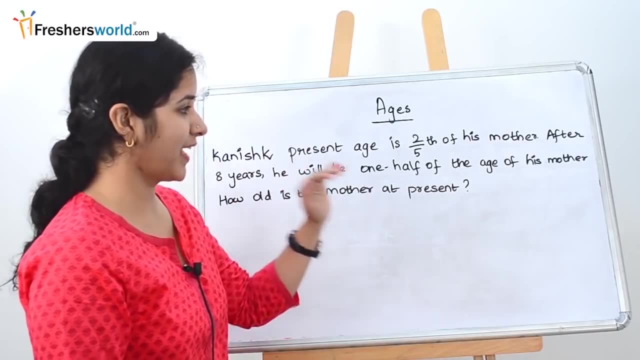 number of years ago. let's solve another problem. okay, the second question that I have given is: Kanishk present age is 2 fifth of his mother. after 8 years he will be one half of the age of his mother. how old is the mother at present? as usual, 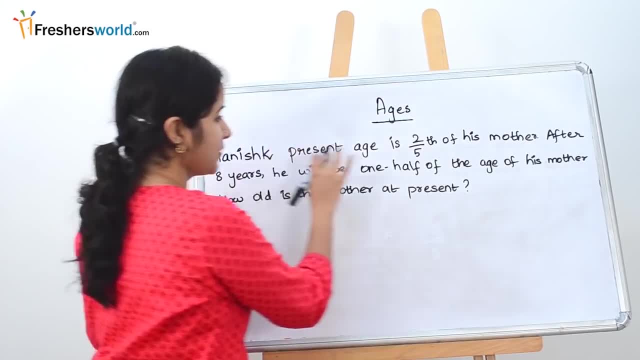 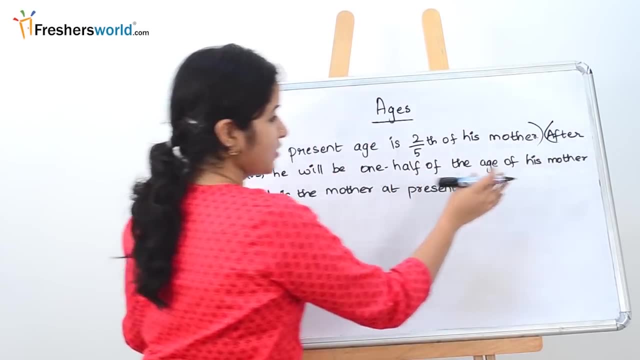 just segregate the question. first part of the question talks about Kanishk. present age is 2 fifth of his mother. second part talks about after 8 years, one half of the age of his mother. and they are asking for the mother's age at present. so let's write it for the first part. they are telling that. let's say: 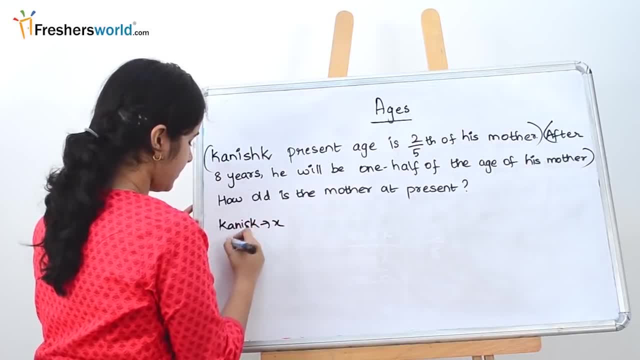 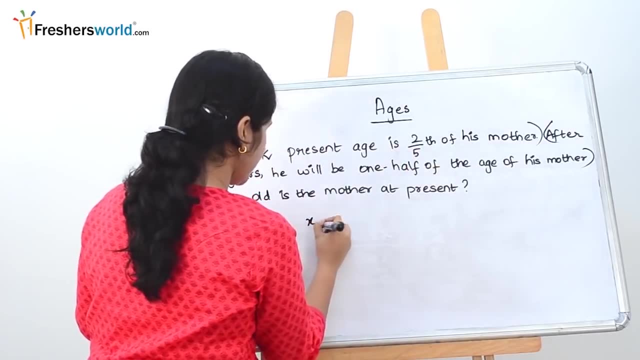 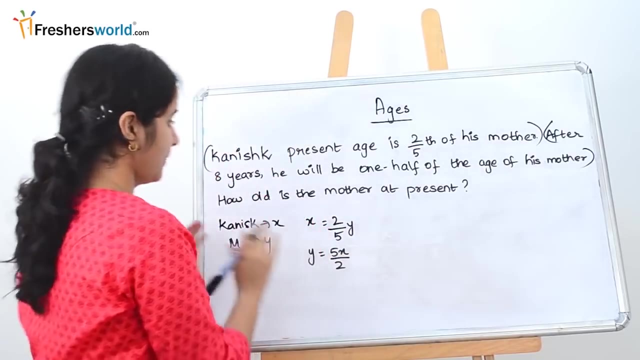 Kanishk age as X and his mom age as Y. so what is the first part? Kanish present age is 2 fifth of his mother. so X is nothing but 2 by 5 of Y. so obviously Y is equal to 5, X by 2. just leave it as such, you know. next, after 8: 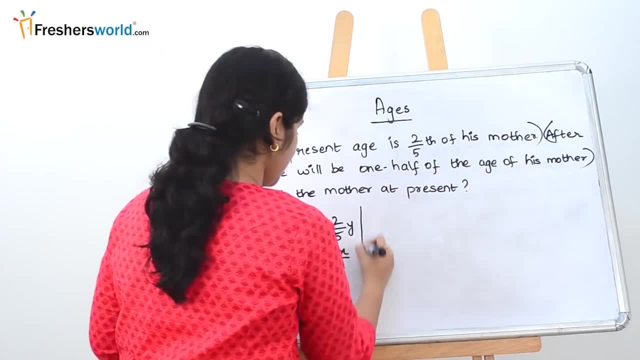 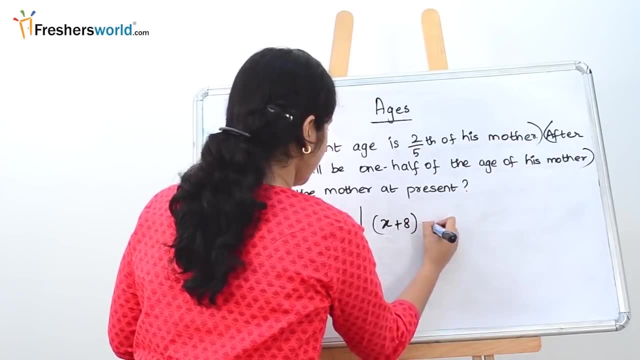 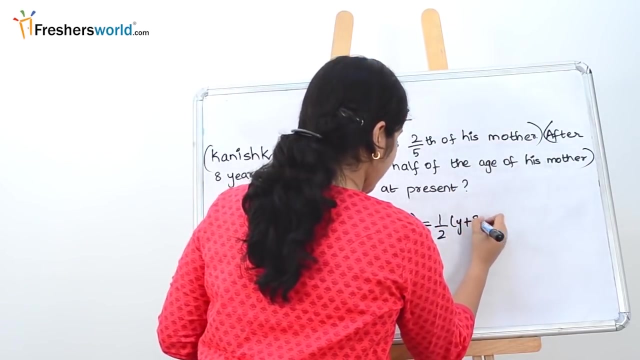 years he will be 1 half of the age of his mother. so after 8 years- the word after means we have to add here- so after 8 years Kanishk age will be 1 half half half of the age of his mother. Mother's age is y, So y plus 8.. So just cross, multiply it 2x plus. 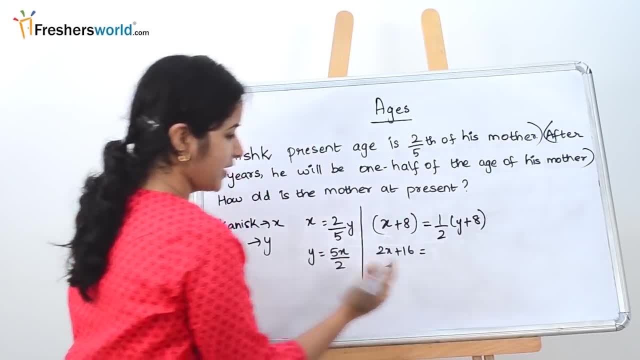 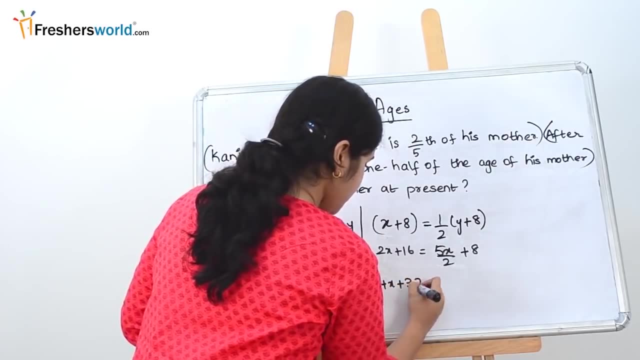 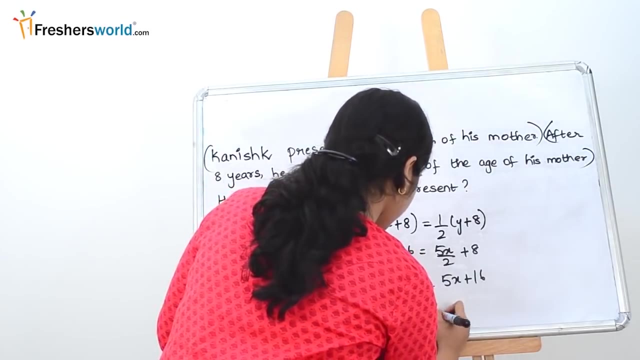 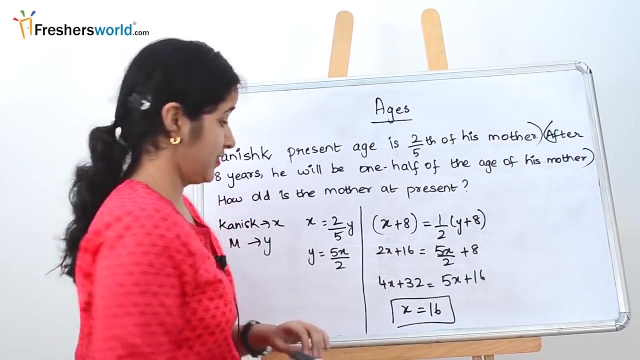 16. y. we can write it as 5x by 2 plus 8. Just cross, multiply 2, again 4x plus 32, 5x plus 16. So take 5x, there x is equal to 16.. So x is equal to 16.. So but read the question. How old is the? 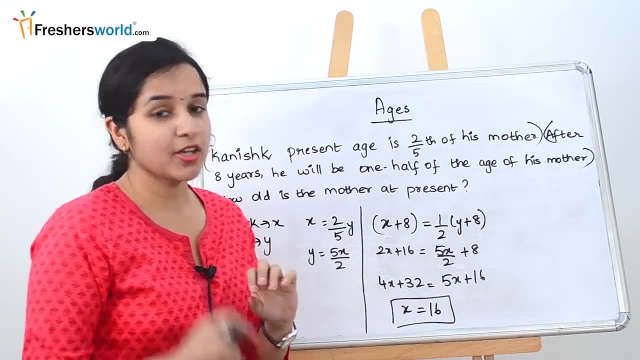 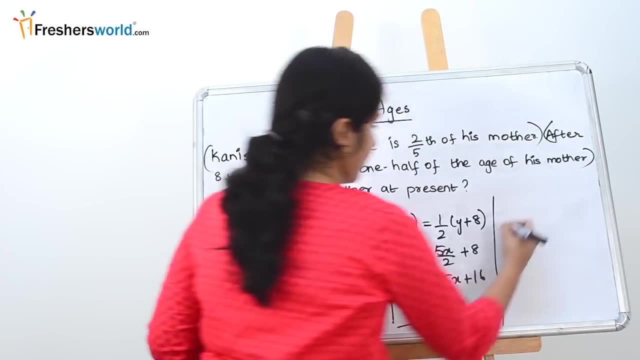 mother at present. So x is nothing but Kanishk age. They are not asking for Kanishk age, They are asking Kanishk mother age. So we know x. now We have to find y. y is equal to 5x by 2.. So 5 by 2. x value is: 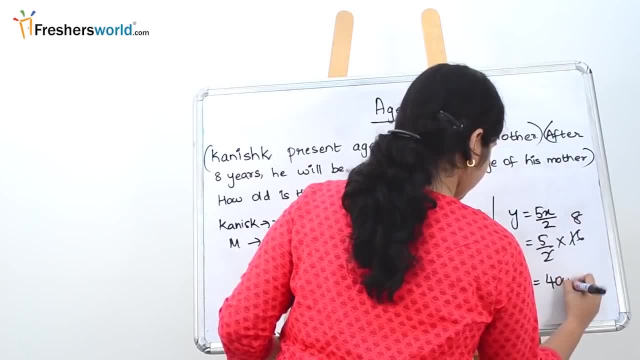 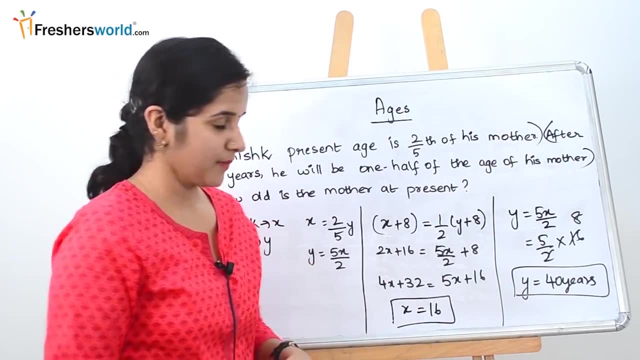 16. So 8, which is 40 years. So mother of Kanishk age at present is nothing but 40 years. This is where the people goes wrong. The question that they have asked is not for Kanishk age. People just stop it. 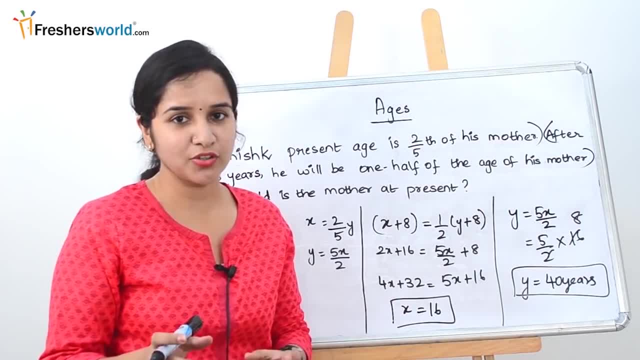 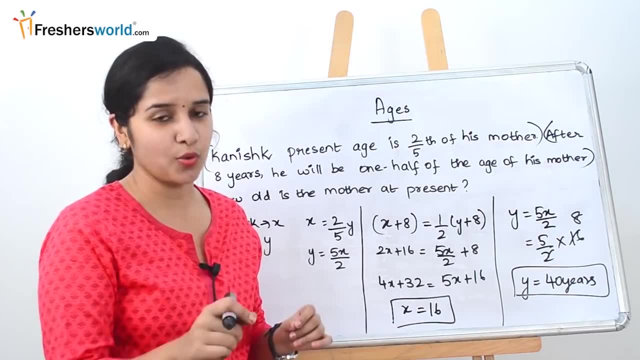 at x is equal to 16, and even in the solution, or answer solution also, you get the option as 16.. So they will directly take it and go to the next question. But read the question carefully. Are they asking for Kanishk age? No, They are asking for his mom's age. So next step you have to solve. 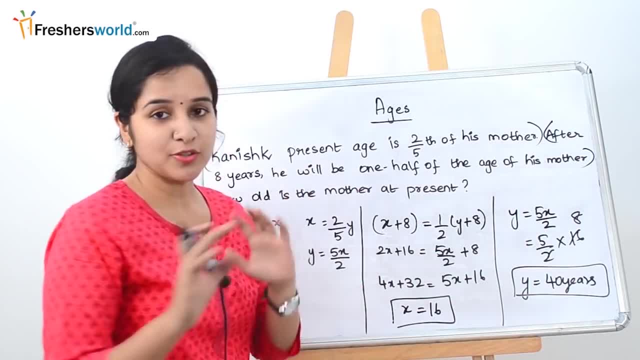 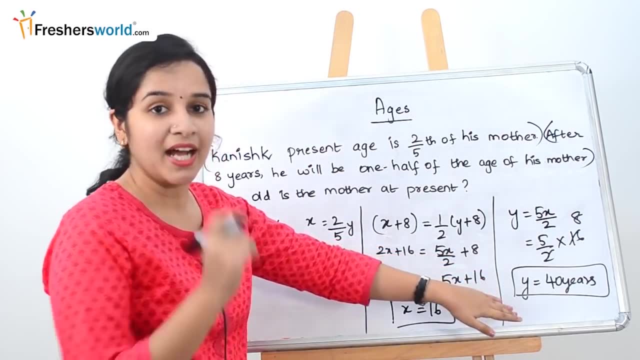 in finding it y to get the 40 years. So that's it. So that's how you have to split the question. First you read the question, Check the equation whether it's pertaining to the question or not. Once you find the answer, again read the question one more time to check whether your answer is pertaining to the question. Let's solve another problem. 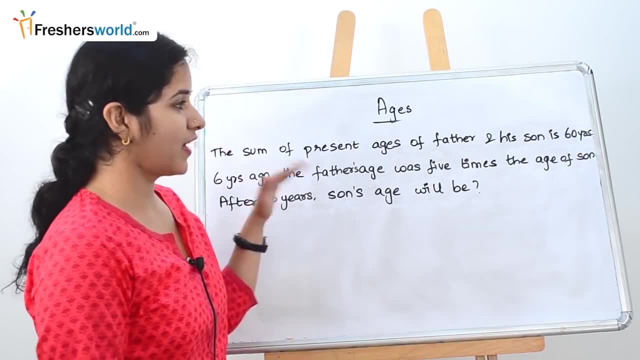 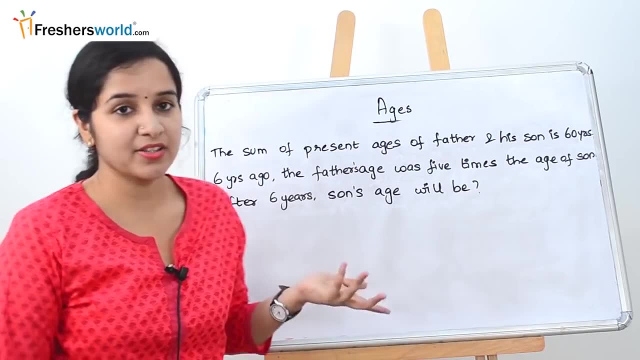 Okay, the next question that they have asked is: some of the present ages of father and his son is 60 years. 6 years ago father's age was 5 times the age of son. After 6 years, son's age will be So. first step, as usual, segregate the question. First part: they are talking about the sum of their present. 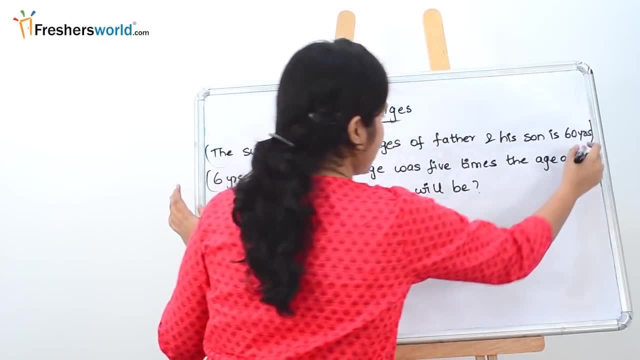 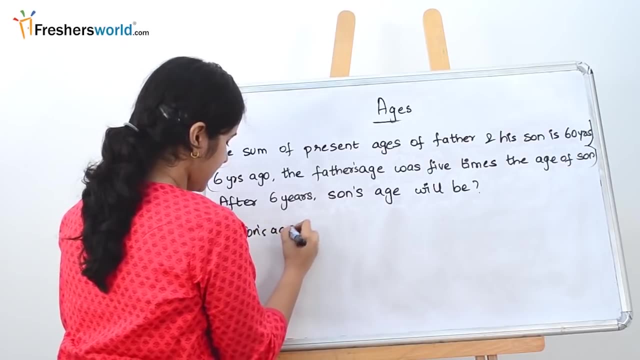 ages, Second part. six years ago, father's age was 5 times the age of son. And then the question they have asked First assign a variable. So let's take sons age as x and father's age as y. Now let's start. 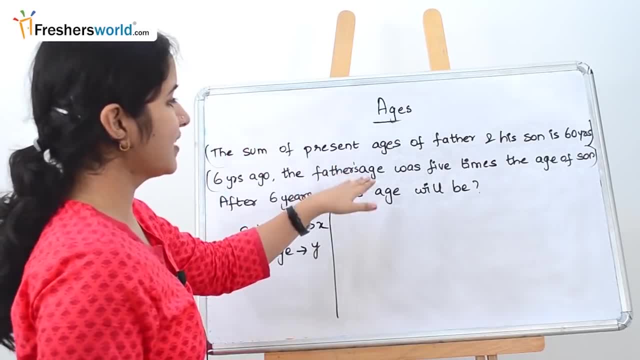 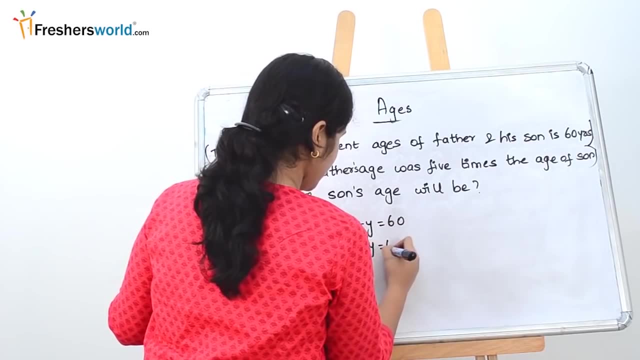 solving the sum. First part talks about sum of the present ages of father and his son is 60 years. So son's age plus father's age is 60. So y is equal to 60 minus 6.. Let's just keep it like that. So the second part of the sum. 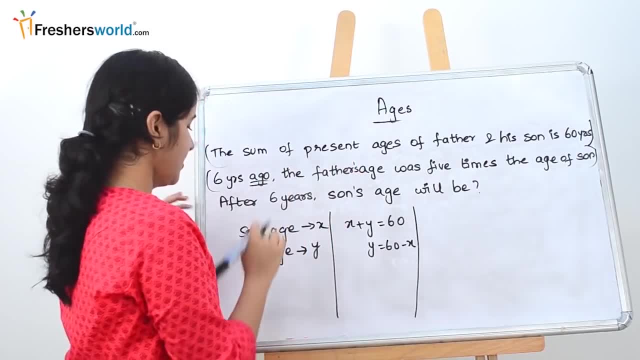 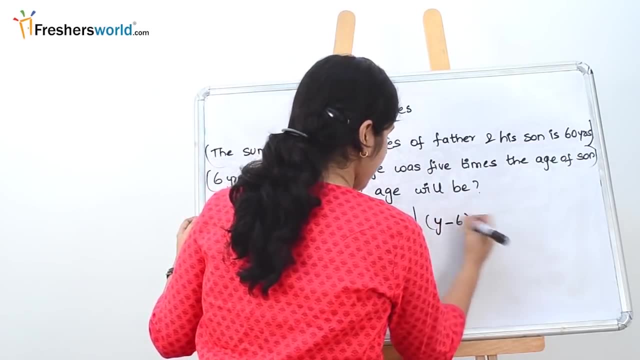 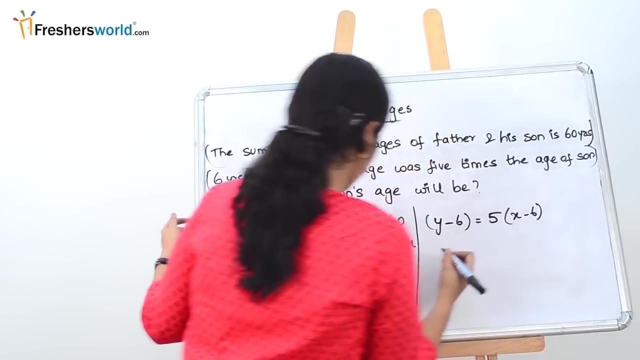 years ago, father's age was 5 times the age of son. So what was father's age? Why? Six years ago ago means we have to subtract it y minus 6.. Father's age was 5 times the age of son. Son is x, so x minus 6.. So we know that y is equal to 60. 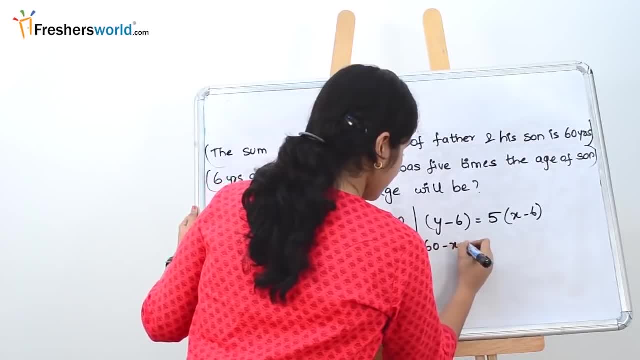 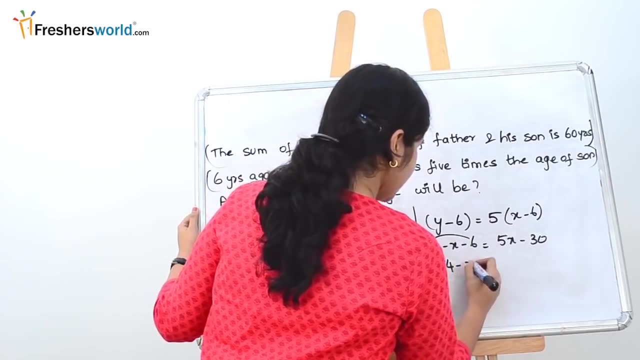 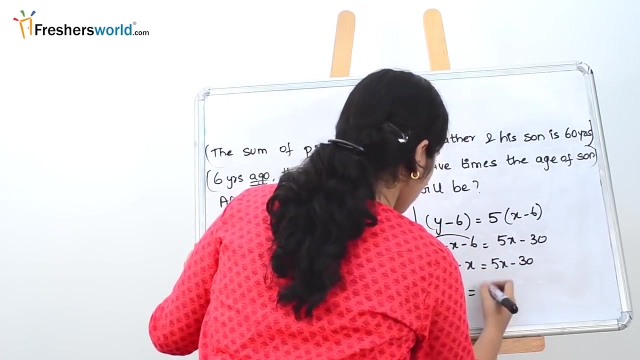 minus x. Substitute it here: 60 minus x minus 6 is equal to 5x minus 30. So 60 minus 6 is 54, minus x is equal to 5x minus 30. So 6x is equal to 84.. 6 ones are. 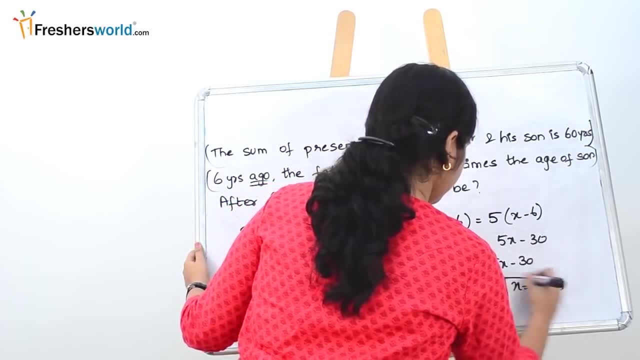 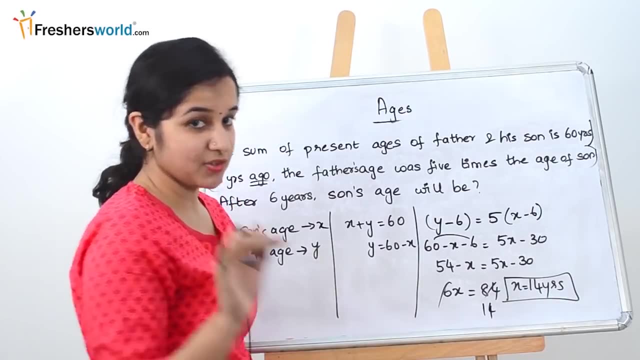 4s. So x is equal to 14 years. So x is nothing but son's age. So son's age is 14 years. Are they asking for the son's age? No, See the question again. After 6 years, what will be the son's age now? 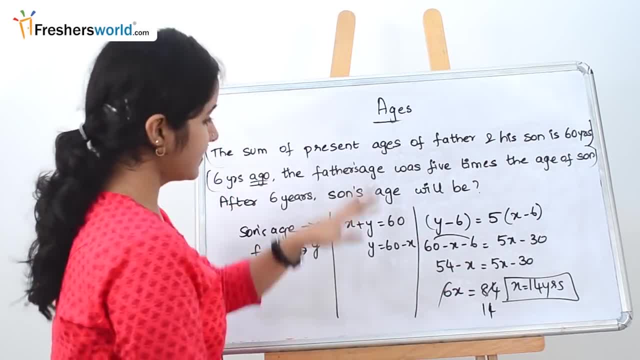 Present age of son is 14.. After 60, 8.. Is he 60?? No, that's again different. And as I have studied for 6 years, 6 years after means is nothing but you have to add. so the present age is: 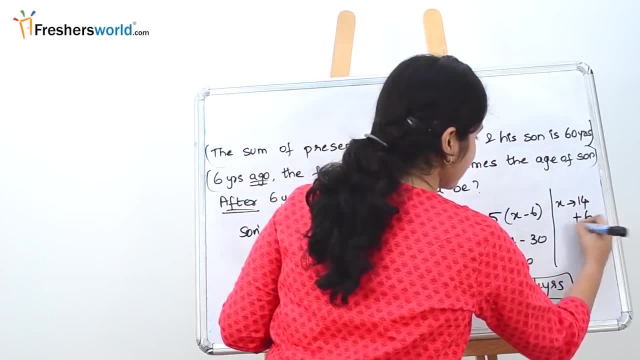 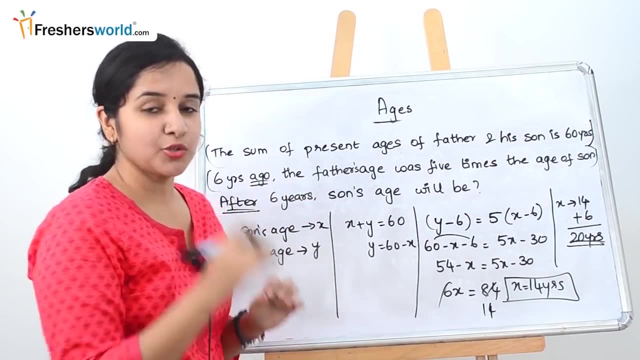 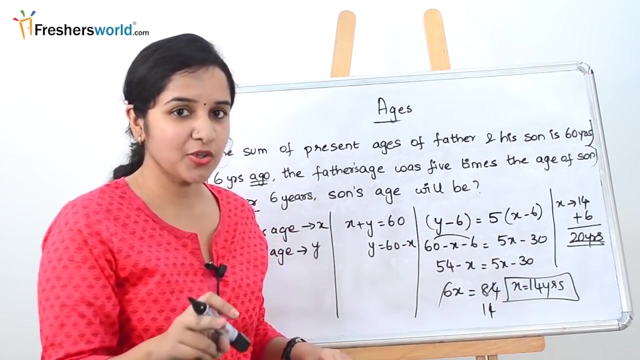 nothing but 14 years after 6 years, so plus 6, so 20 years. as I always say, read your question 2-3 times to understand what they are exactly asking. as for the previous sum, they will also be 14 in your option, but make sure, are they? 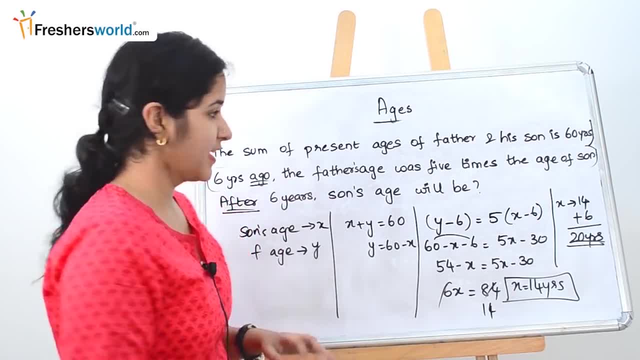 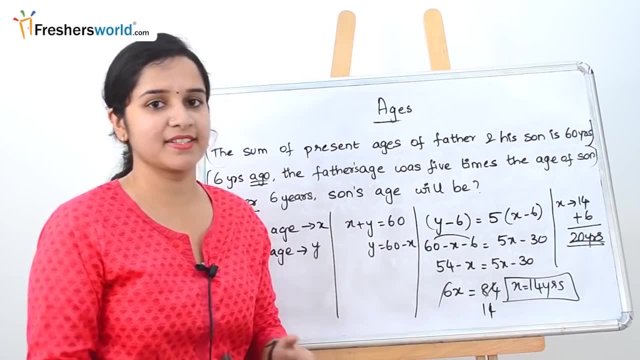 asking for the present age of son, or they are asking for something else. so this is the most common type of ages, some you will see. instead of father and son it will be mother and son or between brother and sister. the same way they will be asking the question. all you have to do is first segregate it, find the 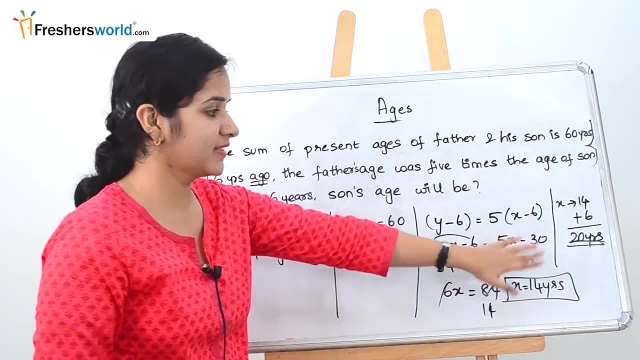 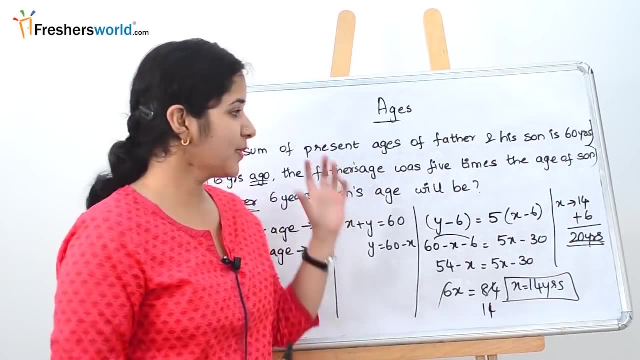 equation for it. substitute the corresponding equation and find the answer pertaining to the what? the question that they have asked in this part of ages we had solved a little bit tougher problems and little bit common problem that you could face in an exam. in the future videos we will be solving. 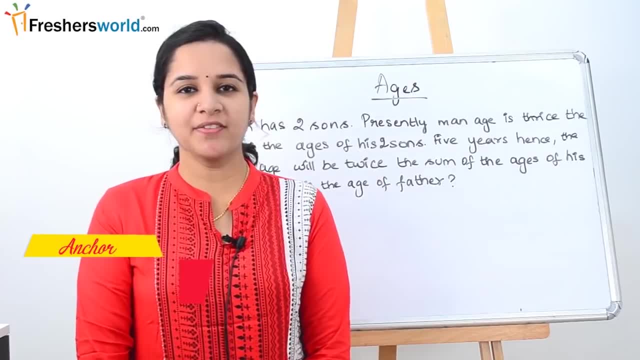 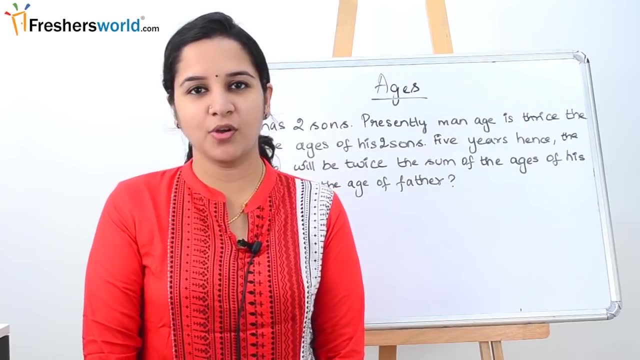 a much tougher problems in ages to understand the concept much better. the topic that we are going to discuss in the next part of the video- so thank you are going to look today- is the ages part 3. in the previous videos of ages we got to know the basic concept of ages and we have solved a couple of simple sums. so 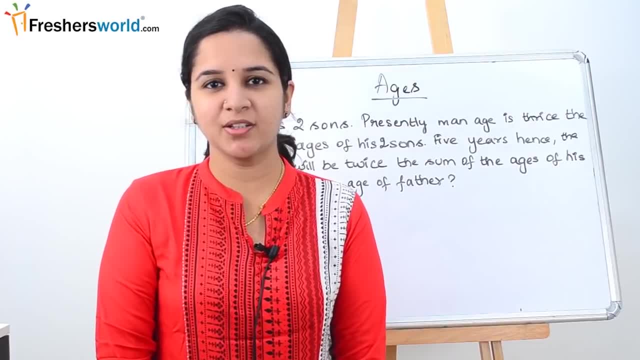 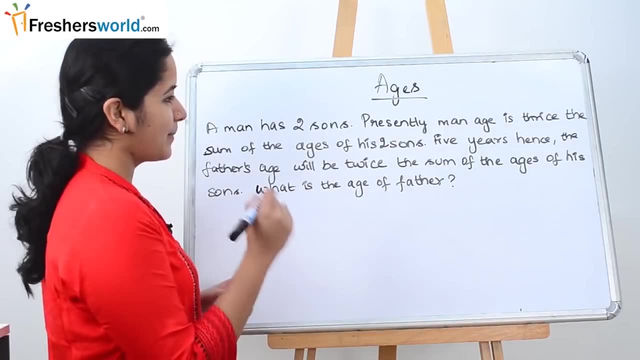 from this part we will be solving a bit tougher problems, to understand the concepts much better and to see what are the problems that you can face in ages. so let's go to the problem, so the question that they have given us. a man has two sons. presently, man's age is thrice the sum of the ages of his two. 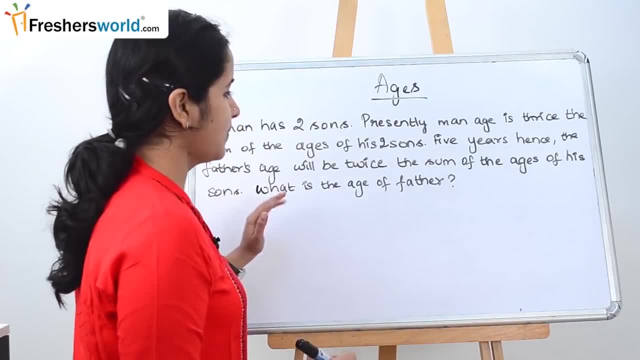 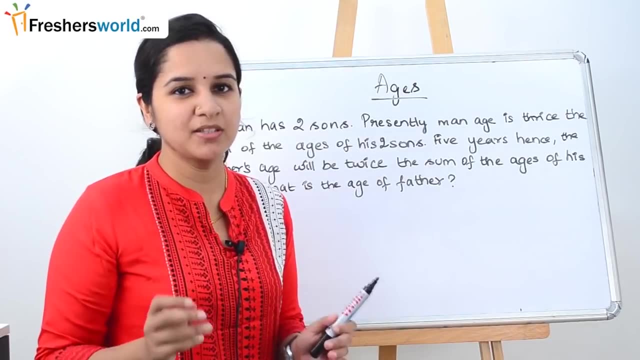 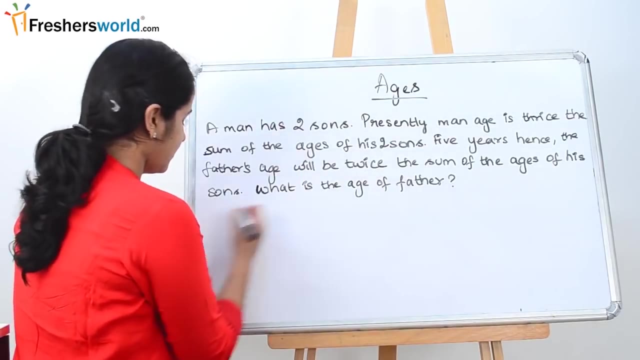 sons five years hence, the father's age will be twice the sum of the ages of his son's. what is their age of the father? so, as I have told you in the previous videos, you have to split the question in the ages to understand it much better. so far they have given. a man has two sons. let's take the father is. 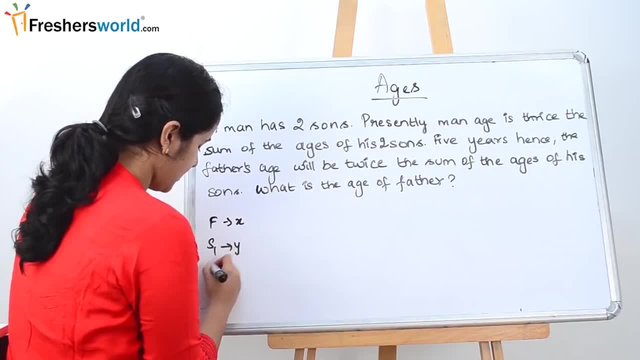 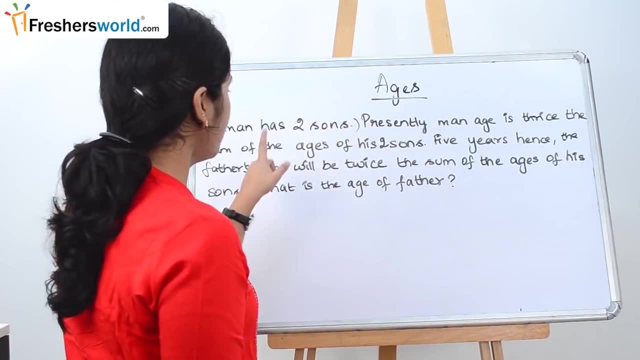 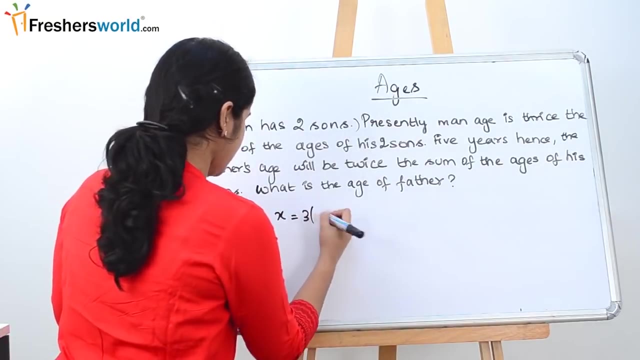 nothing but X, son 1 is white and son 2 is nothing but is it so? this is one part. presently, the man age is thrice the sum of the ages of the son. so present age thrice the ages of his son, which is nothing but 3 of y plus z. 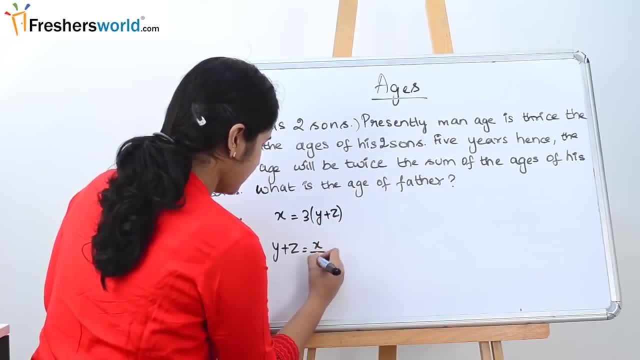 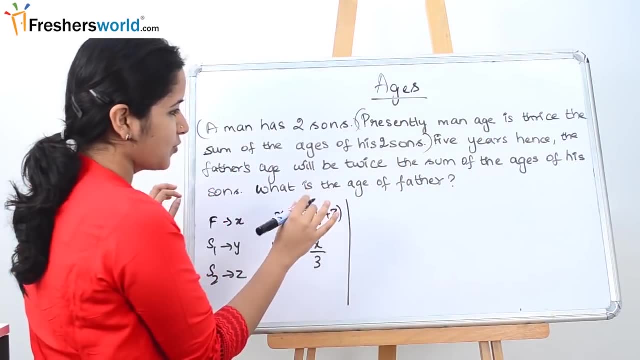 This can be also written as: y plus z is equal to x by 3.. So let's keep it aside. Next part: they have given as 5 years hence, the father's age will be twice the sum of the ages of his sons. 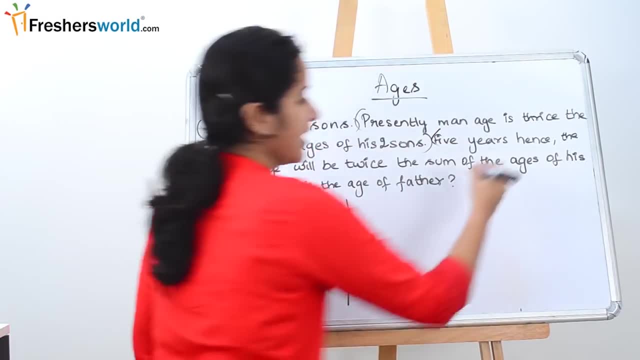 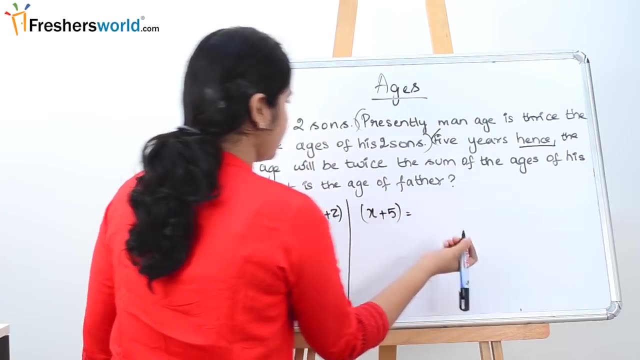 So this is the next part of the question. 5 years hence, Hence is nothing but after 5 years, So plus 5.. So 5 years hence, The father's age will be twice the sum of the ages of his son. 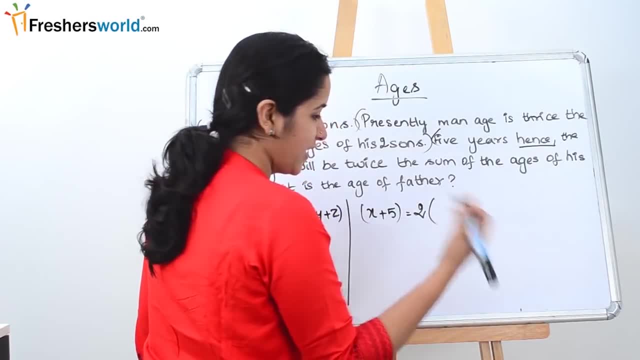 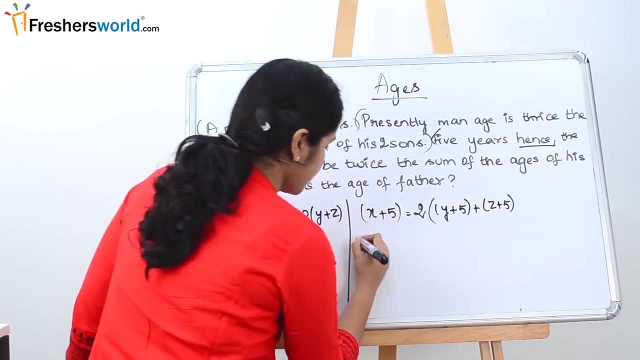 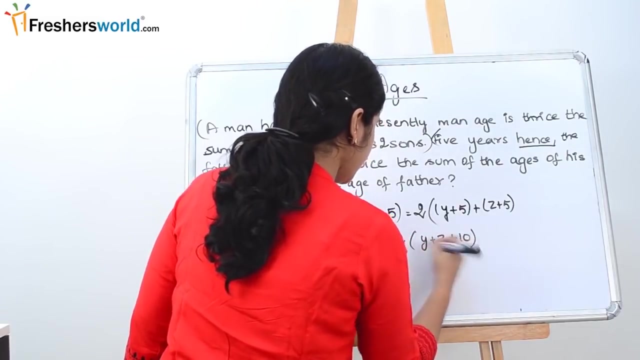 Twice Sons is nothing but ynz, So y plus 5 plus z plus 5.. So let's just simplify it. So x plus 5 is equal to 2 into y plus z plus 10.. So this can be rewritten as x plus 5 is equal to 2.. 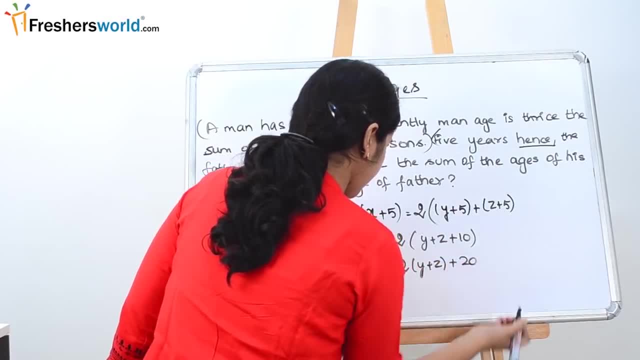 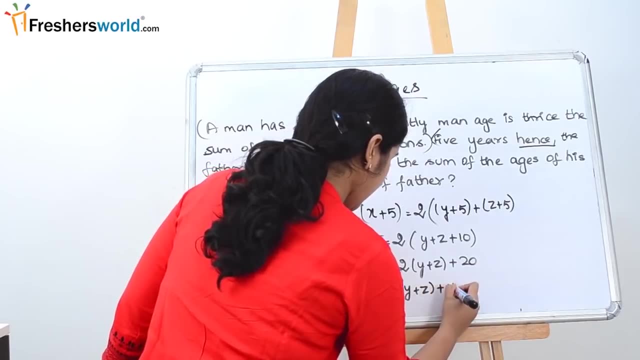 2, y plus z plus 20.. So let's take the 5 that side, So x is equal to 2- into y plus z plus 15.. So we know that y plus z is nothing but x by 3.. 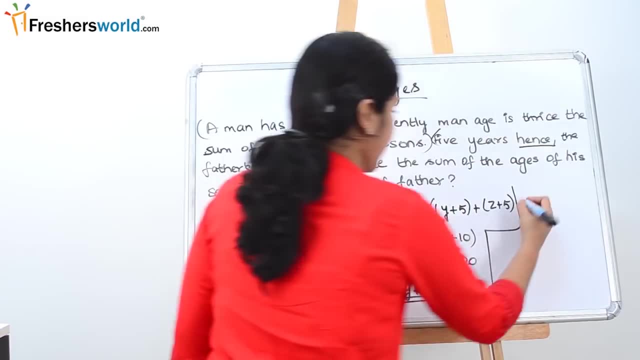 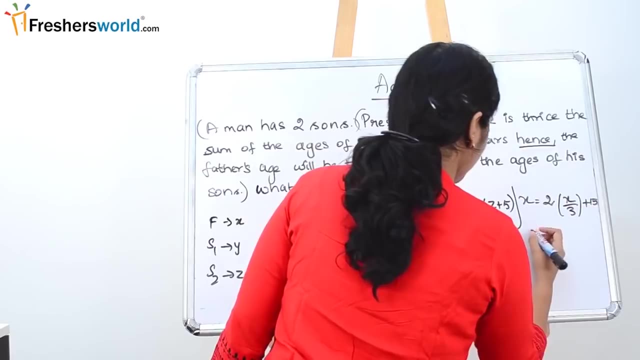 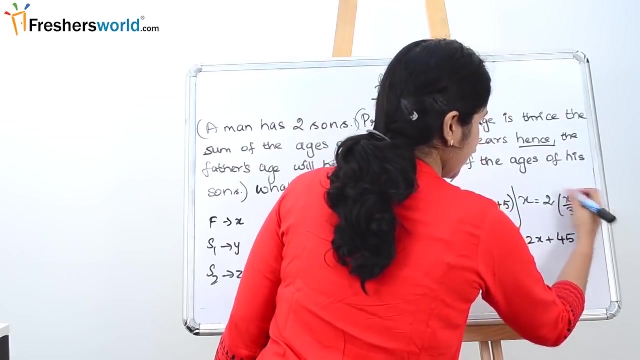 So we are going to substitute it there. So x is equal to 2 into x by 3 plus 15.. So it becomes 3x is equal to 2x plus 14.. So I am cross multiplying it and making it a common denominator. 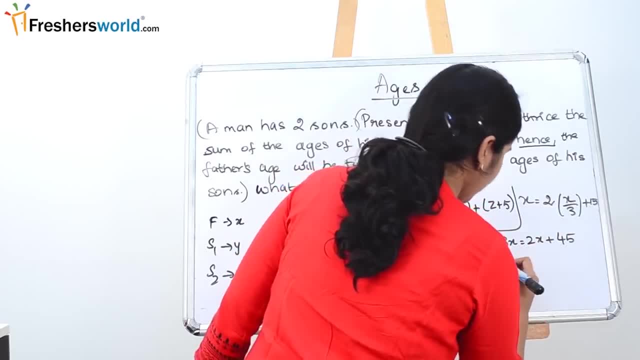 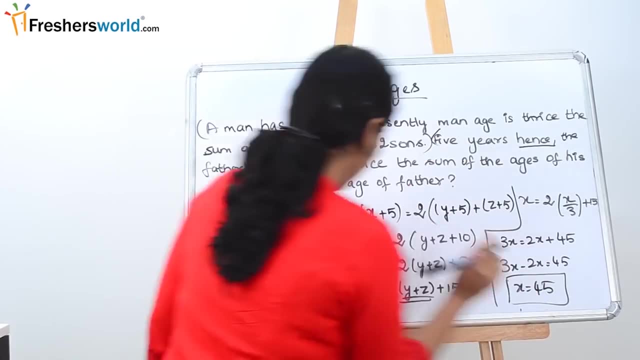 So the 3 goes here, So it becomes 3x is equal to 2x plus 45. So 3x minus 2x is equal to 45 and x is equal to 45. So what is x? x is nothing but father's age. 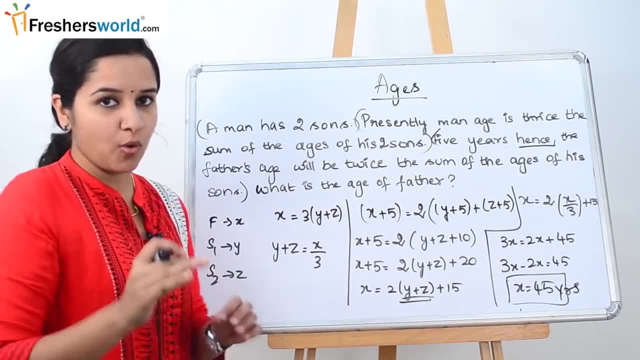 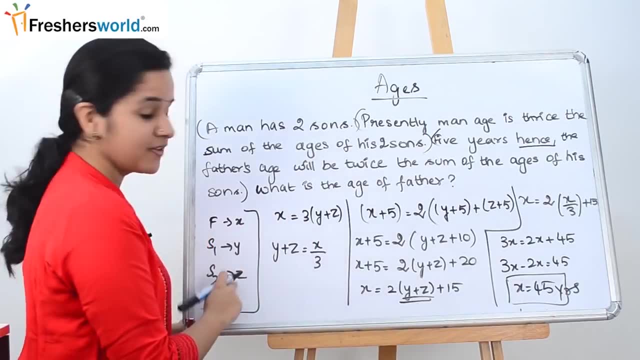 So father's age is nothing but 45 years. So what did we do here? Once we get the question, we split the question, wrote it into 3 equations. First is devising a constant to that. Then first equation, Then the second equation. 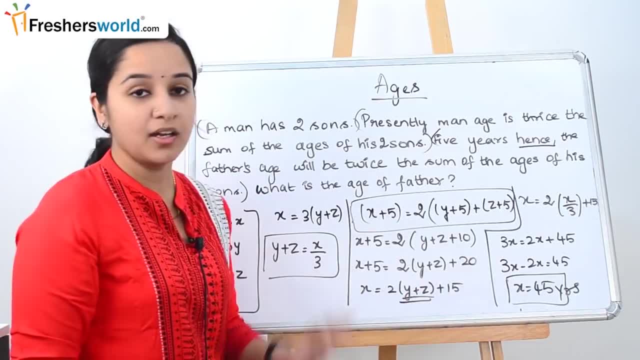 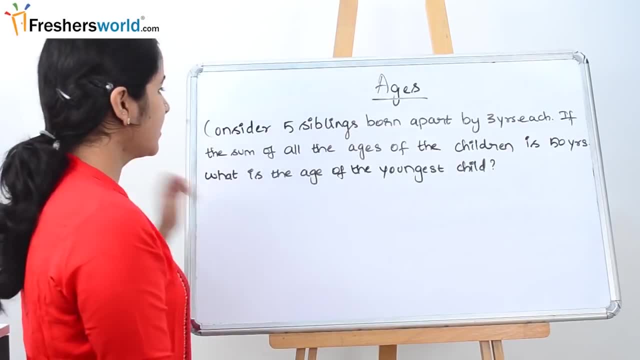 So once you know the equation, it will be very easy for you to find the unknown variable. So let's solve another type of problems to understand the ages concept better. So the next question that they have given is: Consider 5 siblings born apart by 3 years each. If the sum of the ages of the children is 50 years, what is the age of the youngest child? So, as I have told earlier, split the question. Consider 5 siblings born apart by 3 years each. So let's first consider them. 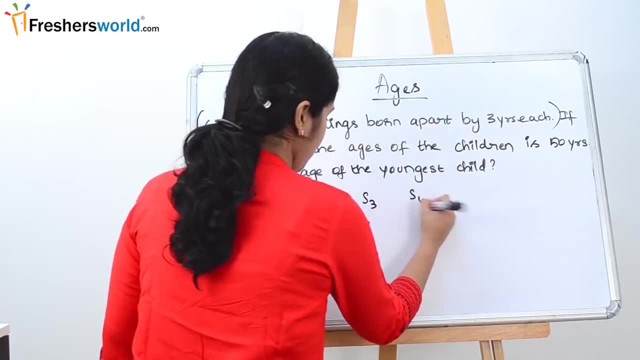 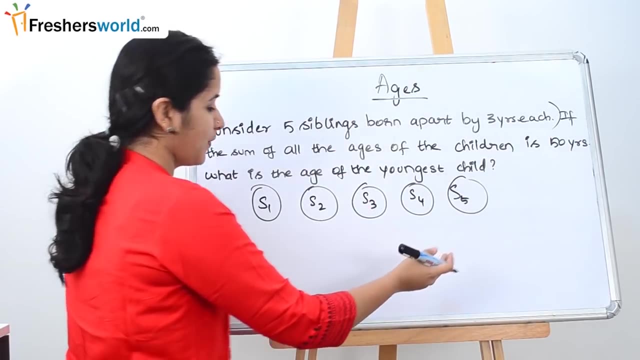 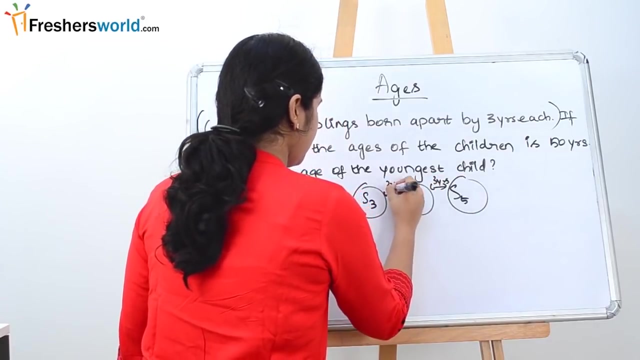 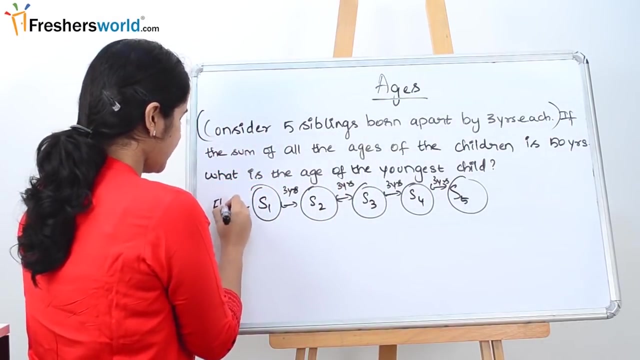 So sibling 1, 2,, 3,, 4, 5.. So they are saying the difference between the siblings is nothing but 3 years each. So each of them has 3 years of difference. Let's check sibling 1 as the eldest and sibling 5 as the youngest. 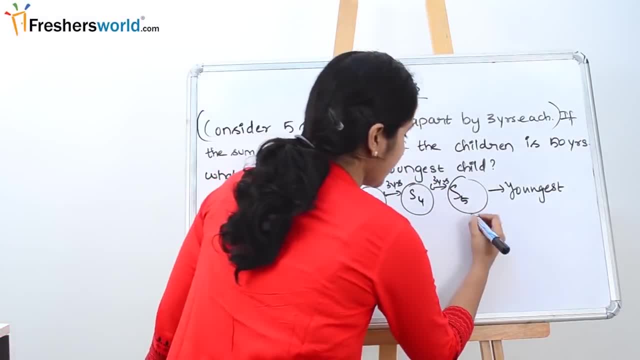 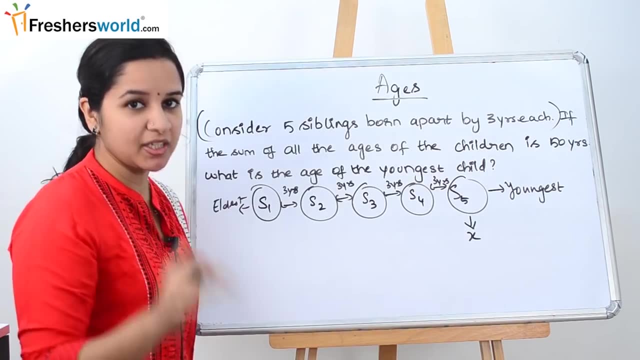 So how to solve this sum? So we know that let's consider sibling 5 as x. We know the difference between the sibling 4 and sibling 5 is nothing but 3 years. So obviously sibling 4 will be 3 years older to sibling 5.. 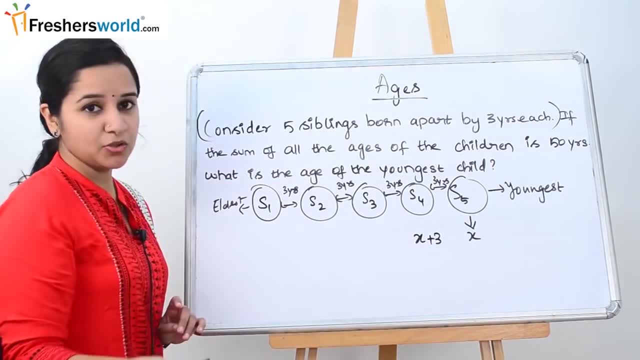 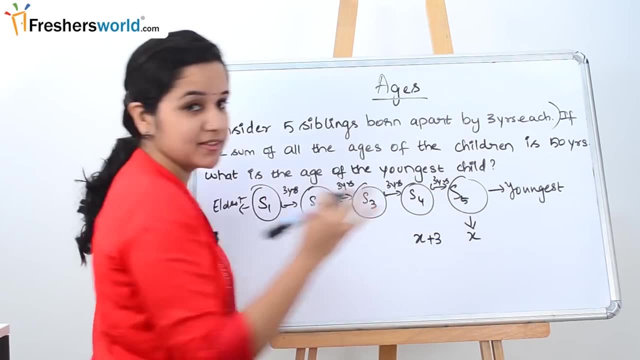 So it will be x plus 3.. So now we consider youngest sibling and the sibling 3. The difference between the sibling 4 and sibling 5 is 3.. And between sibling 3 and sibling 5, sibling 5 is nothing but 6 years. 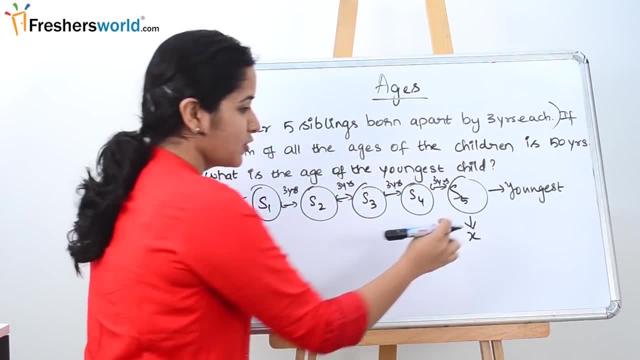 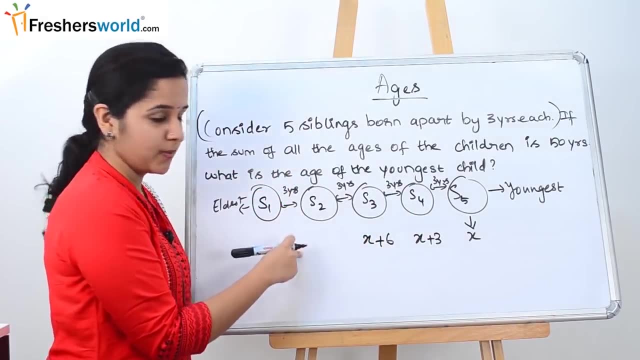 How? Because the difference between each of them is 3 years. So we are adding 3 years of this and then 3 years of this, So it becomes x plus 6.. Now consider the sibling 2. So we know that the difference between them is 3 years. 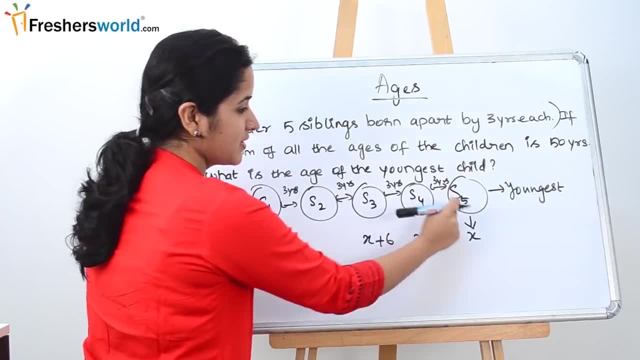 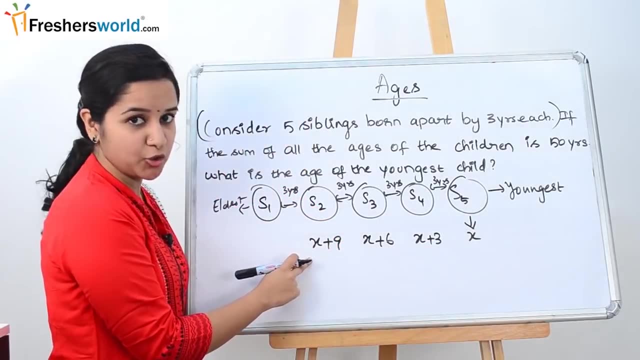 3 years, and 3 years each. So it becomes 3 plus 3 plus 3,, which will be x plus 9.. So sibling 5 is nothing but 9 years younger than the sibling 2.. So let's take sibling 1.. 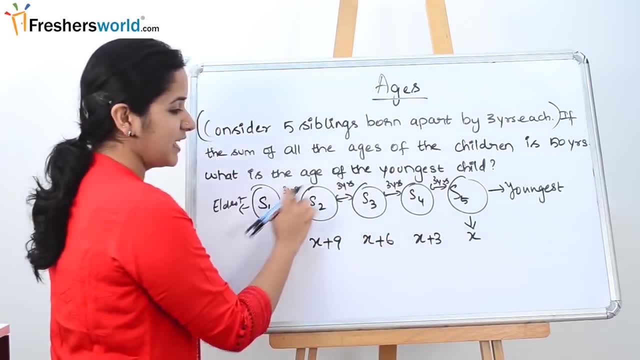 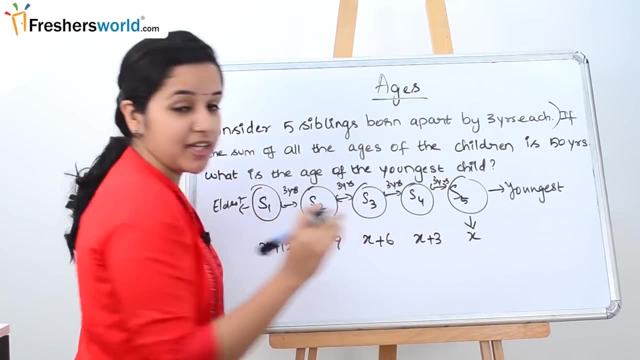 Sibling 1 is nothing but the addition of all these years, Which is nothing but 3 plus 3 plus 3 plus 3.. Which is nothing but x plus 12.. So what are these? So we have considered sibling 5 as x. 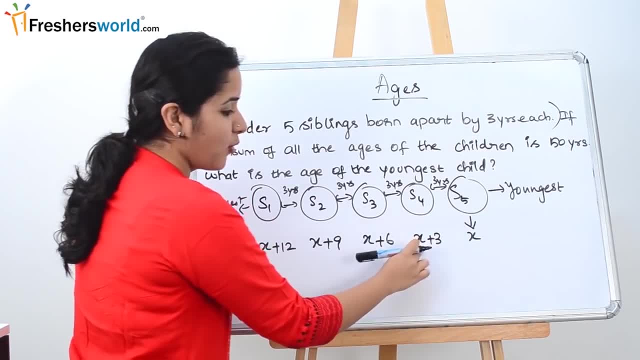 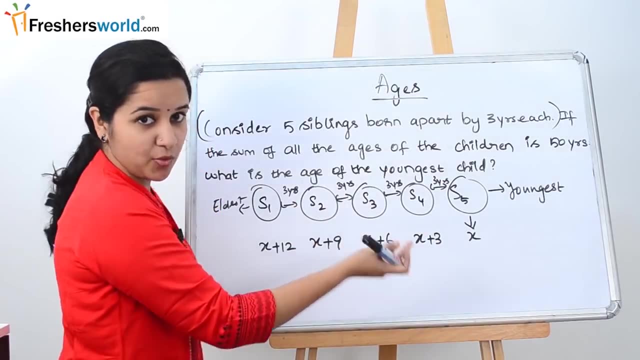 And we are seeing the age difference of each of them. So sibling 4 is 3 years older than x, Sibling 3 is 6 years older than 5.. And sibling 2 is 9 years older And sibling 1 is 12 years older. 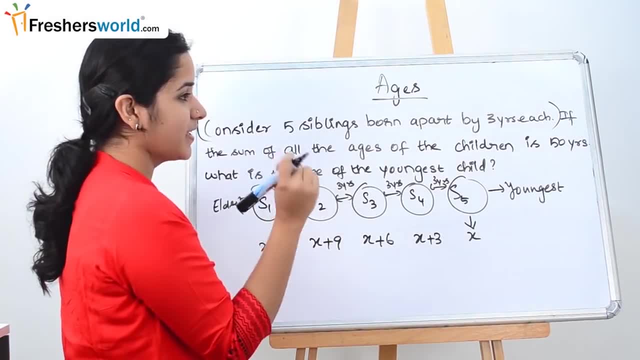 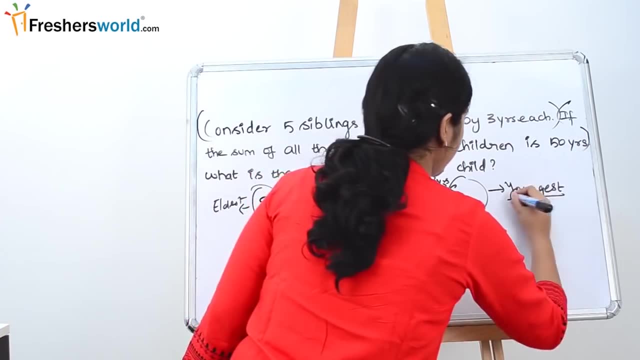 Let's go to the next part of the question. If the sum of all the ages of the children is x, then the sum of all the ages of the children is 50 years. What is the age of the youngest child, So we have to find, is nothing but the youngest child. 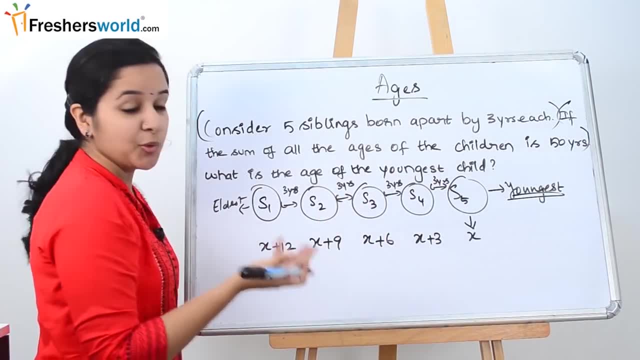 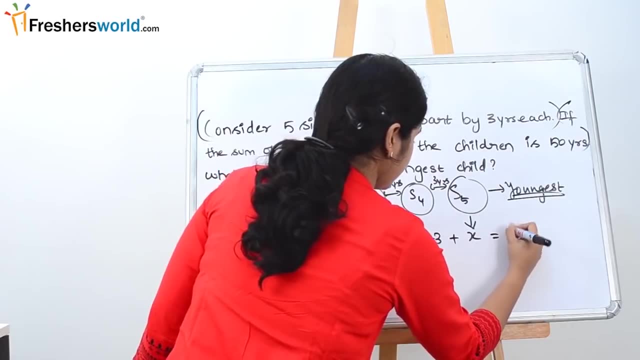 Now they are asking: sum of all their ages is 50 years, Which is nothing but addition of all this is going to be 50 years, So add it So 1,, 2,, 3,, 4, 5.. 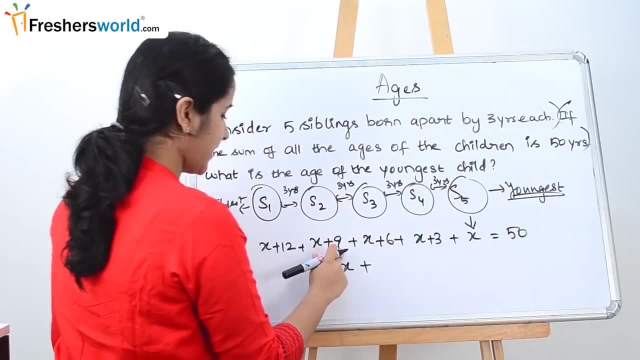 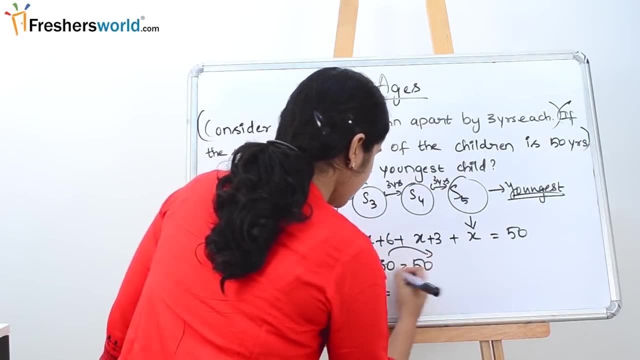 So 5x plus 12 plus 9 is 21.. 27 is 30. It is equal to 50.. 5x is equal to 30. We are taking that side, 50 minus 30 is 20.. 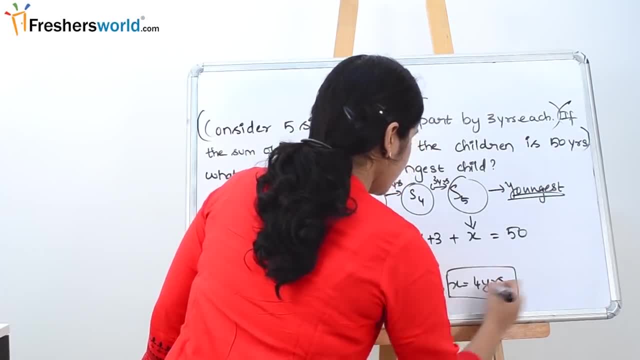 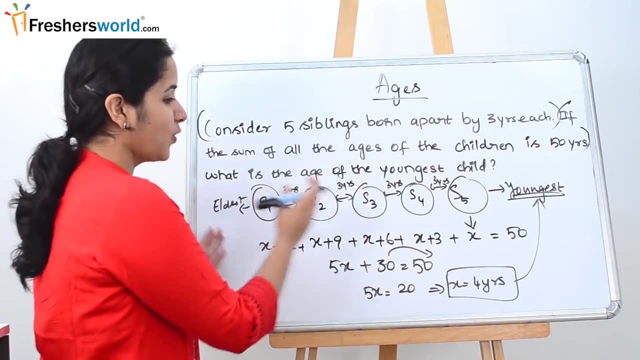 And x is equal to 4 years, So the age of the youngest child is nothing but 4 years. So what did we do in this question? First we split it across, Then we wrote the 5 siblings And we found the age difference between them. 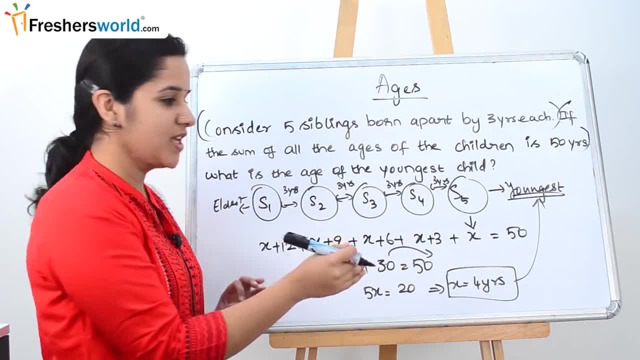 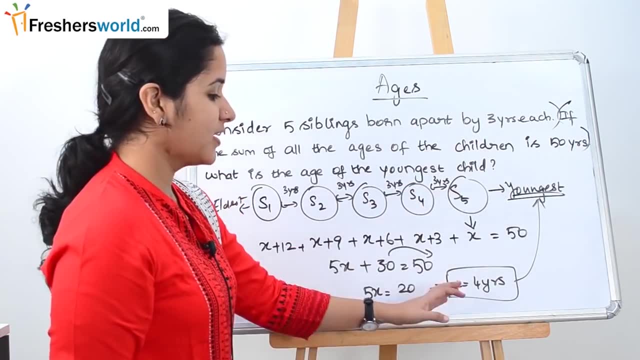 Second part of the question told addition of all these ages is 50. So we equated it to 50 and find the unknown variable x. x is nothing but the youngest child age. So we know the youngest child age is 4 years. 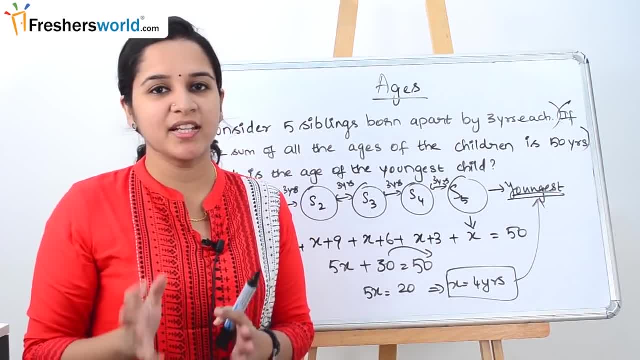 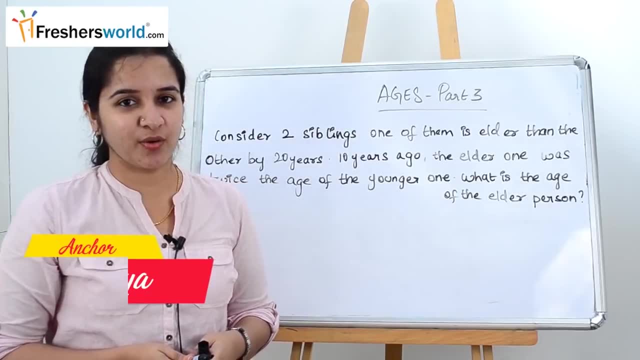 In this video we discussed about two different sums to understand their concept better. In the upcoming videos we will be solving much tougher problems on ages to understand this concept overall better. The topic that we are going to look today is ages part 3.. 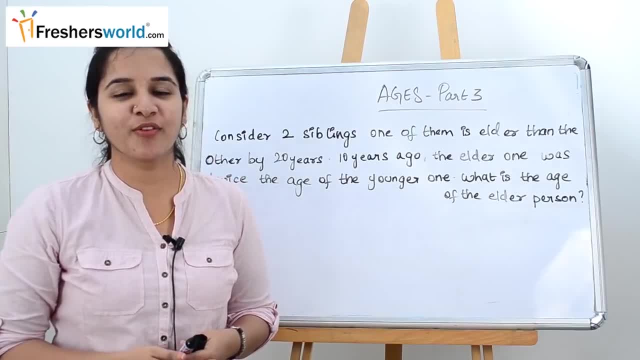 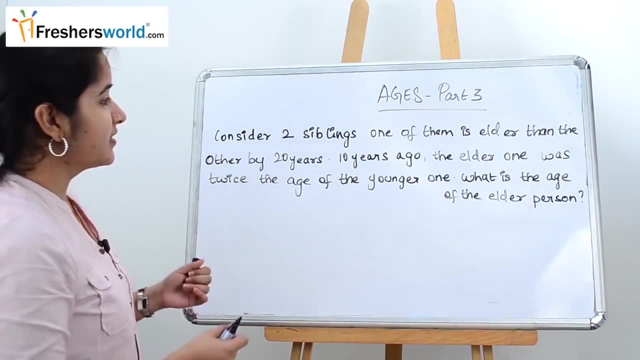 So in the previous parts of ages we dealt with the simpler sums. Going forward, we have to solve tougher problems to understand the overall concept of ages better. So let's get started. The question that they have given is: Consider two siblings. 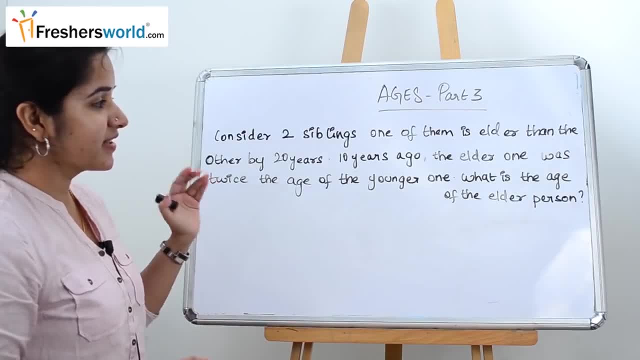 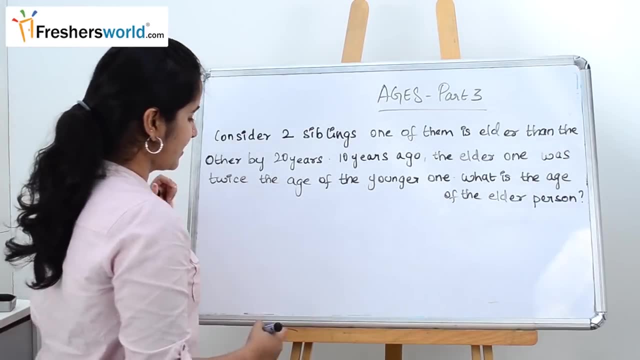 One of them is elder than the other by 20 years. 10 years ago the elder one was twice the age of the younger one. What is the age of the elder person? So there are two siblings. Let's take x and y. 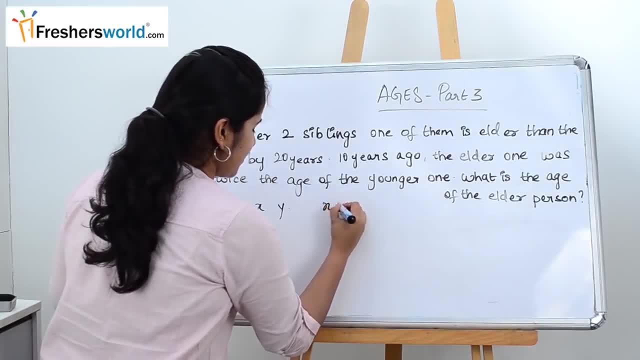 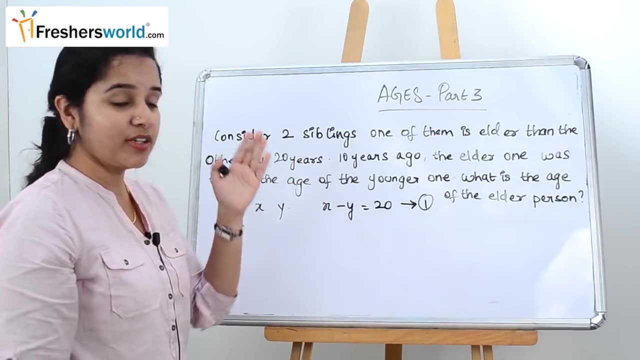 One of them is elder than the other by 20 years. So first equation they have given is: x minus y is 20.. So consider this as a funny equation. 10 years ago, before 10 years, the elder one was twice the age of the younger one. 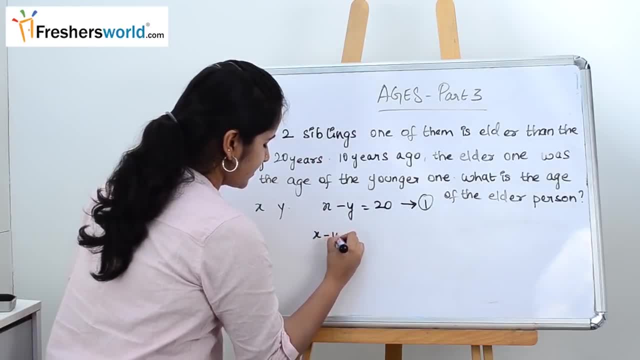 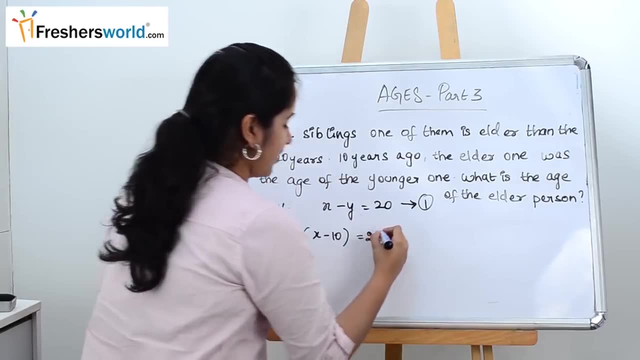 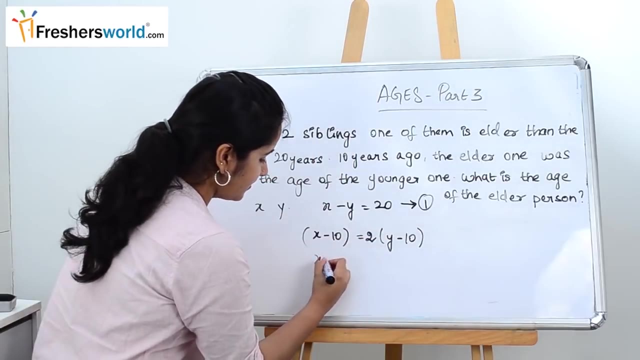 10 years ago, So x minus 10.. 10 years ago the elder one was twice the age of the younger one, So the younger one will also be 10 years below. So this is your second equation. Let's solve this. 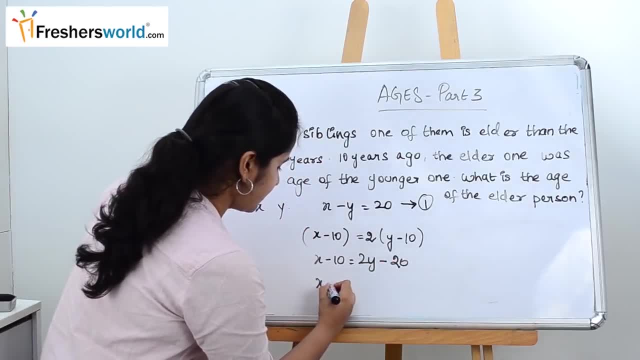 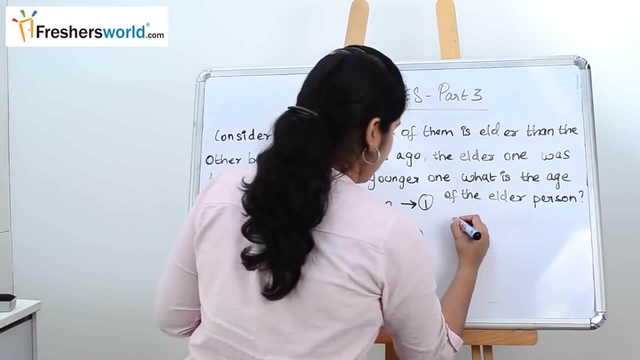 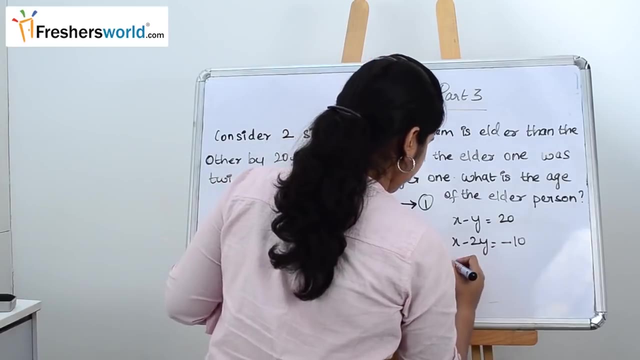 2y minus 20.. So x minus 2y becomes minus 10.. So we know the equation 1 and equation 2.. So x minus y is equal to 20.. x minus 2y is equal to minus 10.. 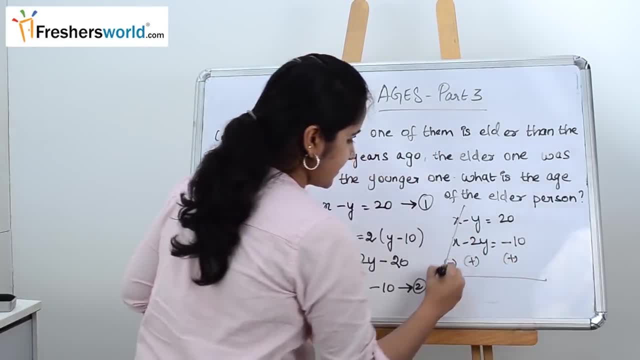 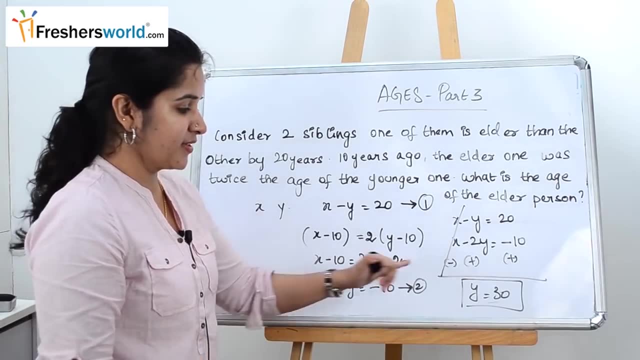 So let's solve this. xx gets cancelled, This becomes y, So y is equal to 30. So y is nothing but your younger sibling. So are they asking that in the question? No, What is the age of the elder person? 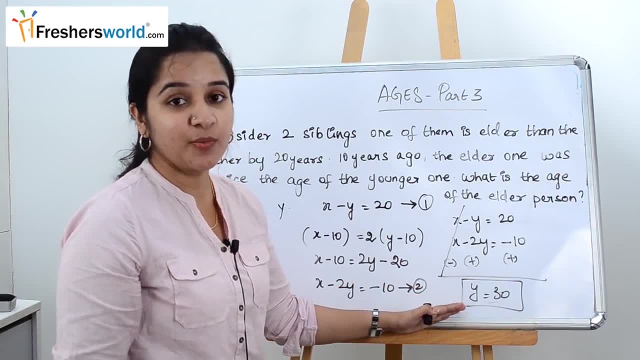 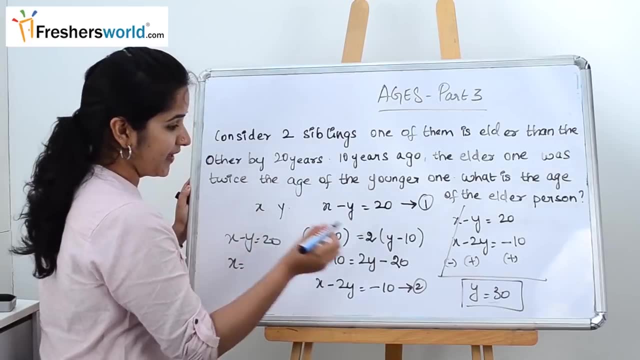 So now we know the age of the younger one Elder is nothing but 20 years elder to him. So nothing but x minus y is equal to 20.. So x is equal to y is nothing but 30 goes, that side becomes 50.. 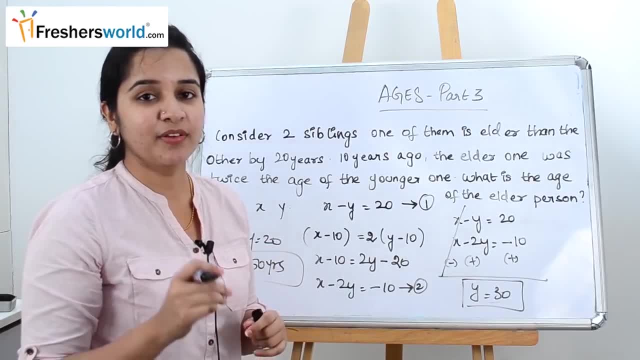 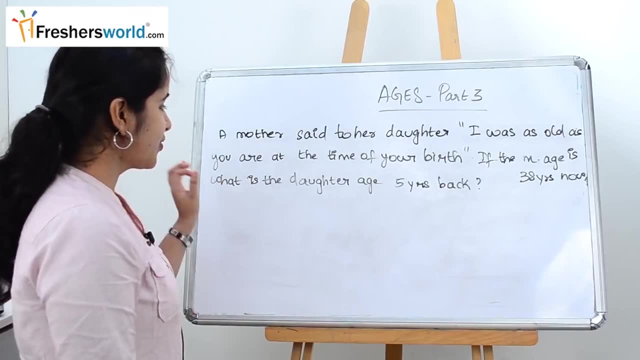 So the age of the elder sibling is nothing but 50 years. So let's go to the next question. The next question is: a mother said to her daughter: I was as old as you are at the time of your birth. If mother's age is 38 years now, what is the daughter's age 5 years back? 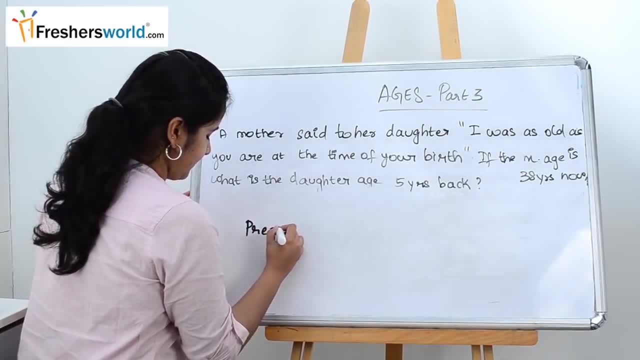 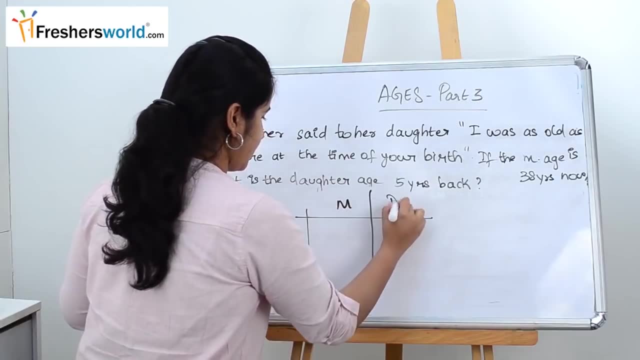 So let's take it as two equations: At present and at the time of daughter's birth. So mother's age is 38 years now. So mother's age and daughter's age. So currently we know that mother's age is nothing but 38 years. 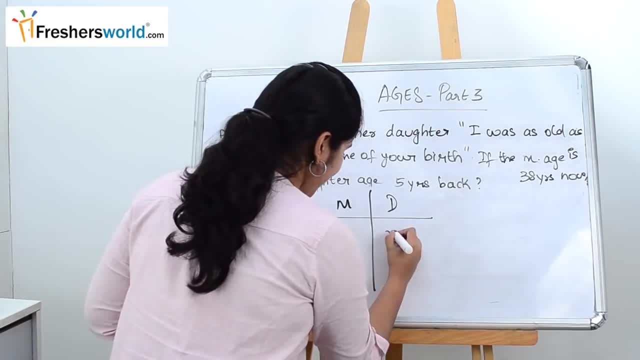 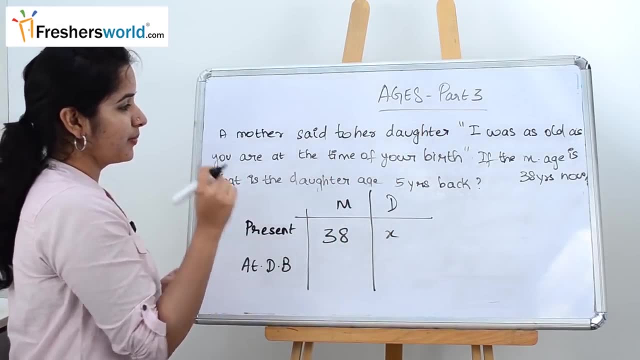 So we don't know the age of daughter, So let's keep it as x. So at the time of daughter's birth, So what she has told I was as old as you are at the time of your birth. 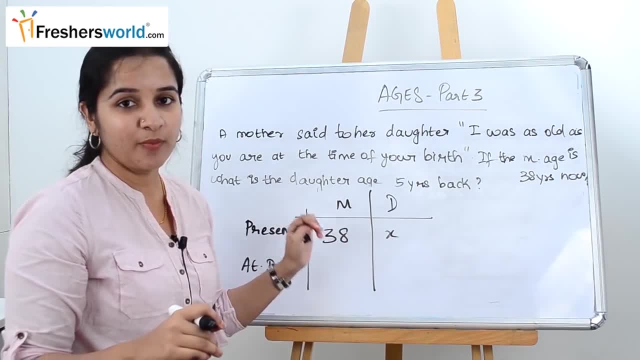 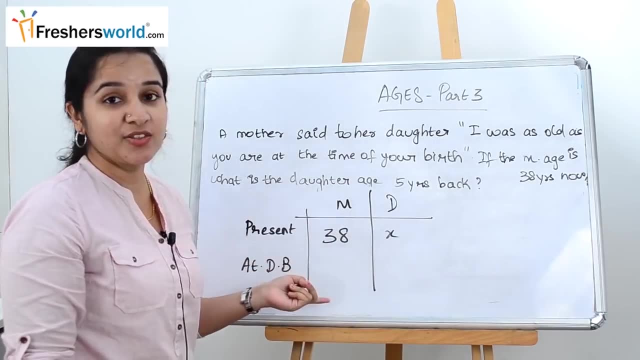 So, whatever the present age of daughter, that's what her mom was when she was born. So basically, let's take a daughter's age may be 20 years or something, So the mother's age will be the same At that time. 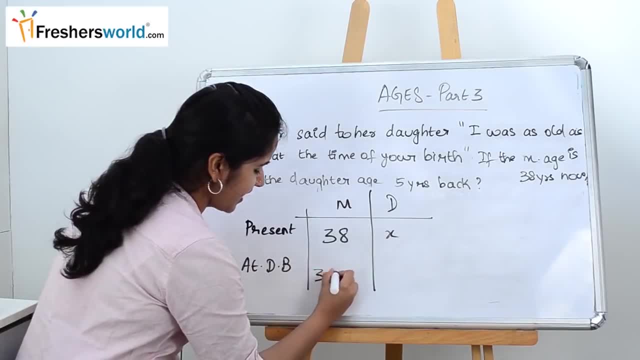 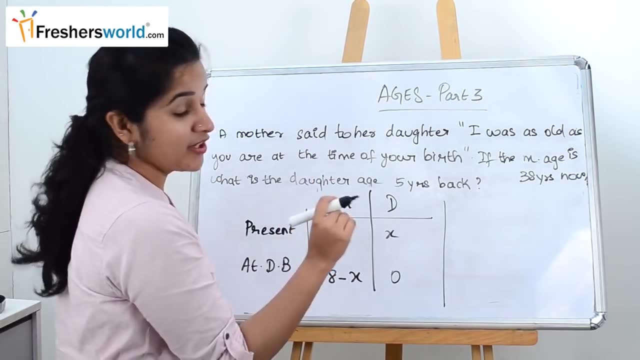 So we don't know the age, So we take it as x. So here it will be 38 minus x, So daughter's age at her birth will obviously be 0.. So leave that. So let's go back to the question and read it again. 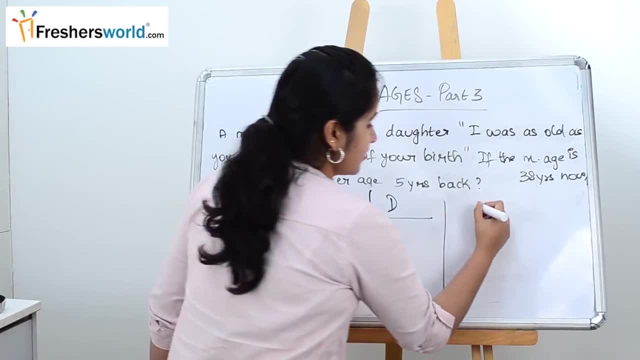 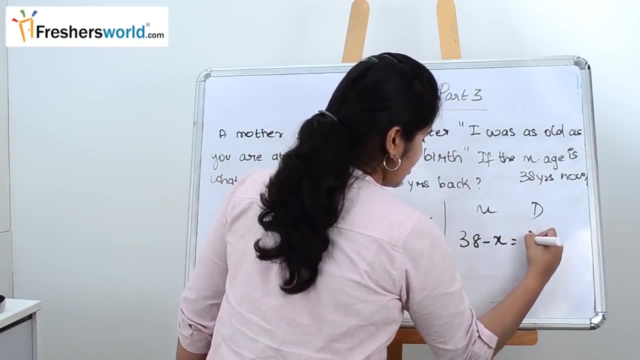 I was as old as you are at the time of your birth. So mother, daughter, we have to form an equation to find the answer. So mother will be 38 minus x, which is equal to x. This is the equation that we are forming from this sentence. 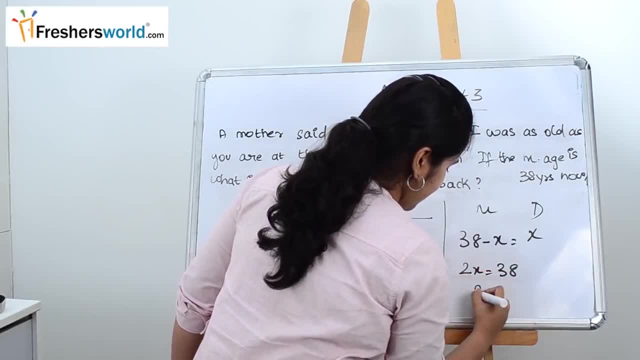 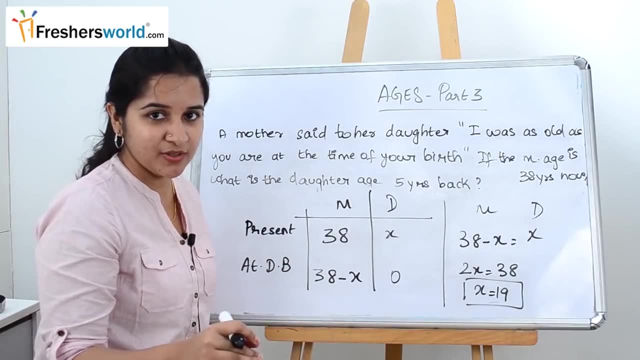 So take x together, 2x becomes 38 and x is equal to 19.. So the current age of the daughter is nothing but 19.. Are they asking you the current age of the daughter? No, They are asking you what is the daughter age 5 years back. 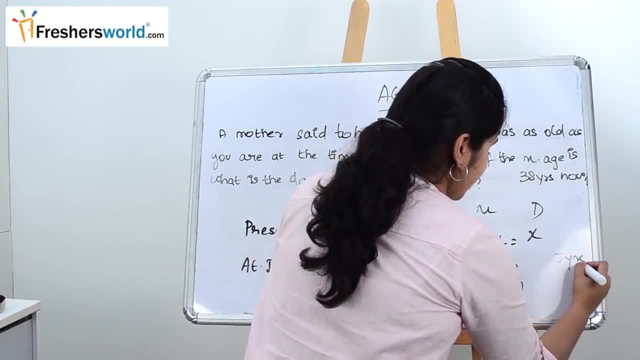 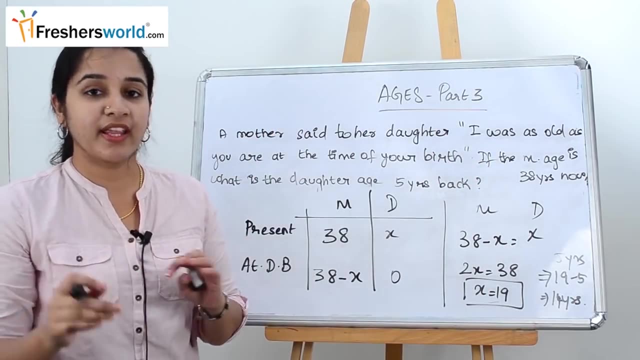 So currently she is 19.. So 5 years back is nothing but 19 minus 5 is nothing but 14 years. So they will twist you and ask you different type of question. If they are going to ask you, the current age of daughter is 19.. 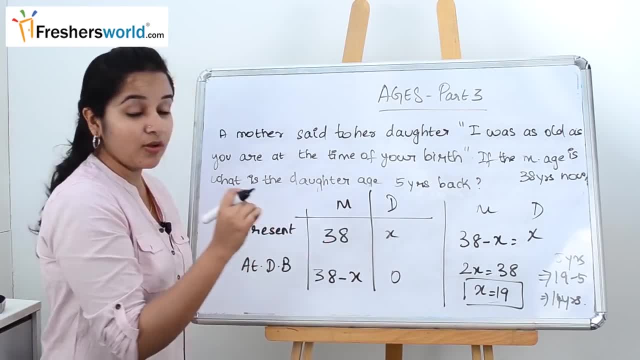 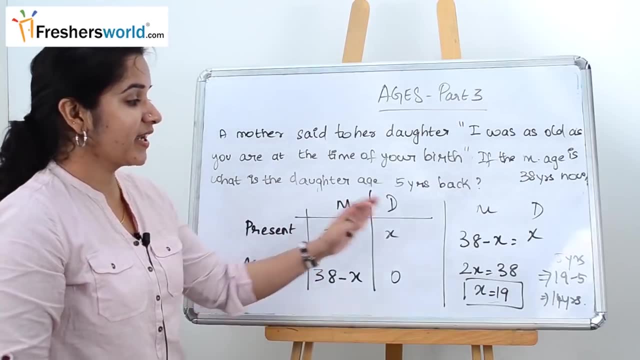 5 years back. you know it is 14.. They might also ask you what is the age of the mother during the daughter's birth, Which is nothing but 38 minus 19.. So various kind of question can be asked in this format. 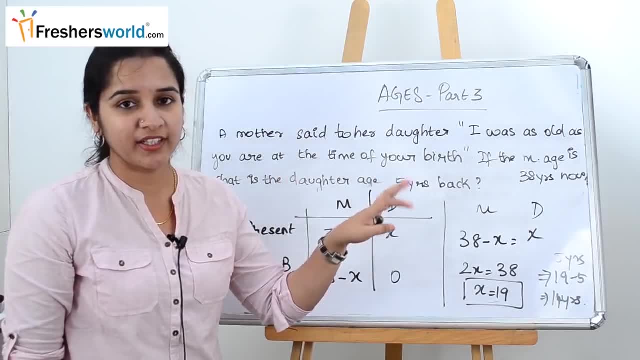 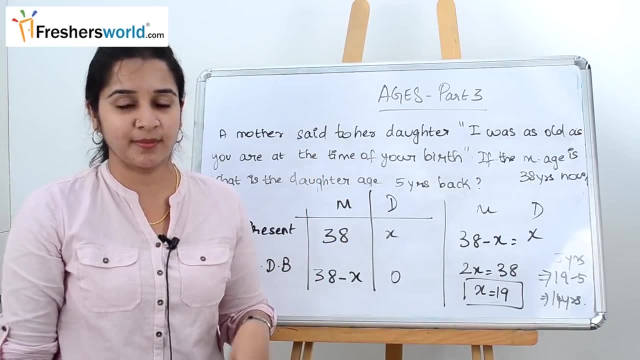 And they can also change. instead of mother and daughter It can be father and son or various other relationship that can be asked. So this is the most common type of problem that you can face in the aptitude exam. Let's go to the next question. 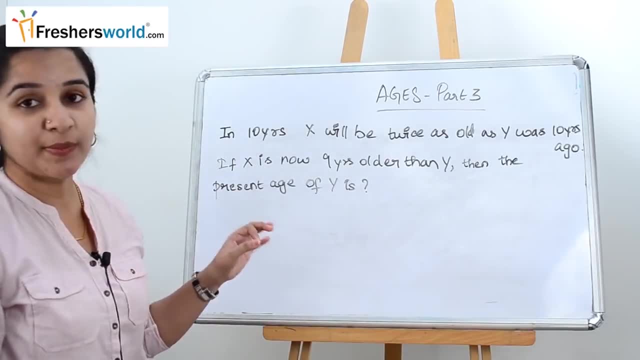 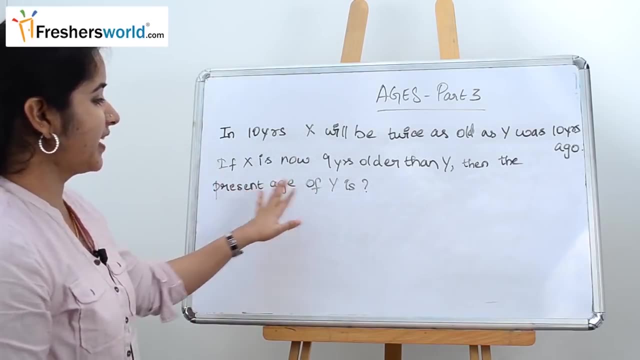 So the next question is: in 10 years, x will be twice as old as y was 10 years ago. If x is now 9 years older than y, then the present age of y is, So it is a classic question that you can face in ages. 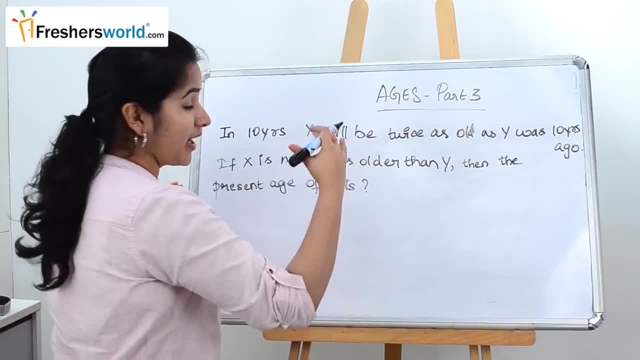 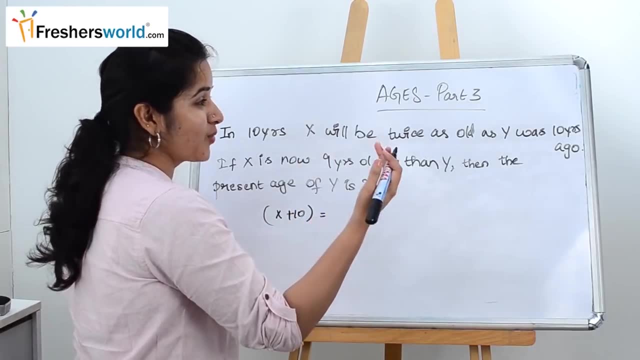 Let's write the first equation In 10 years, So after 10 years, So x will be So x plus 10.. He will be twice as old as y, Twice as old as y 10 years ago. 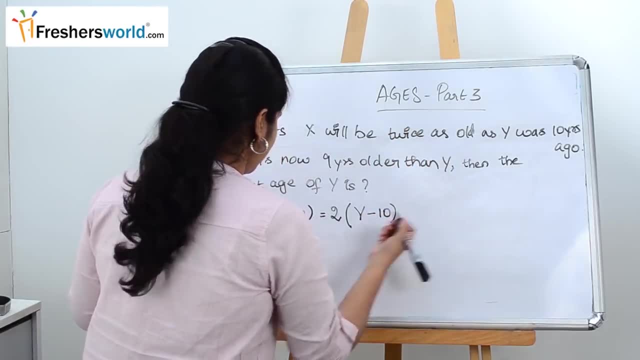 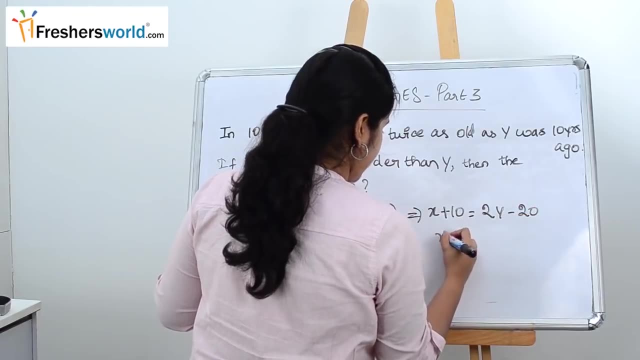 So before 10 years, So minus 10.. So it can be simplified and written as x plus 10. Which is equal to 2y minus 20.. x minus 2y is equal to minus 30. So this is one equation. 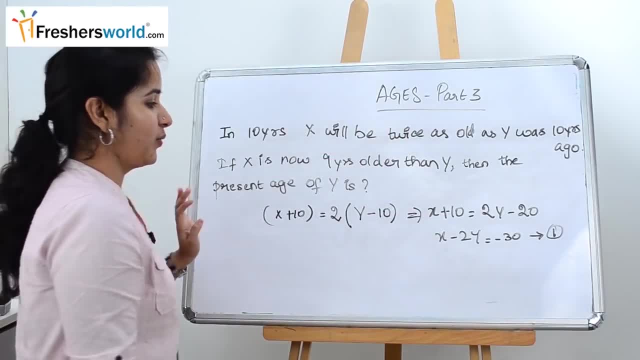 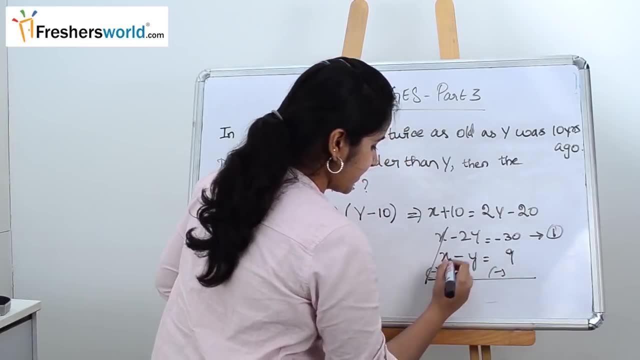 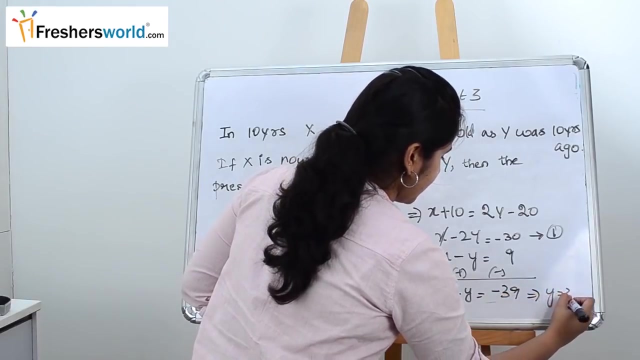 What is the second equation? x is now 9 years older than y, So x minus y is equal to 9.. So let's solve this. xx gets cancelled, It becomes minus y is equal to minus 39.. So y is equal to 39.. 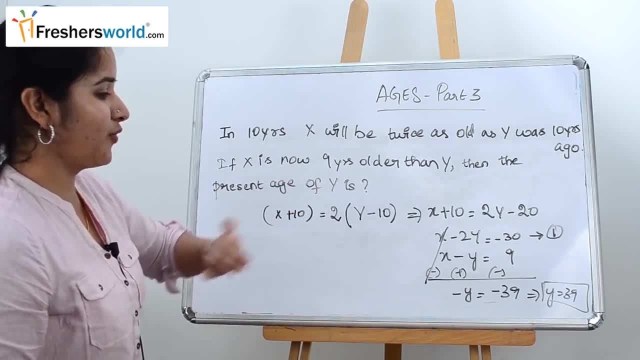 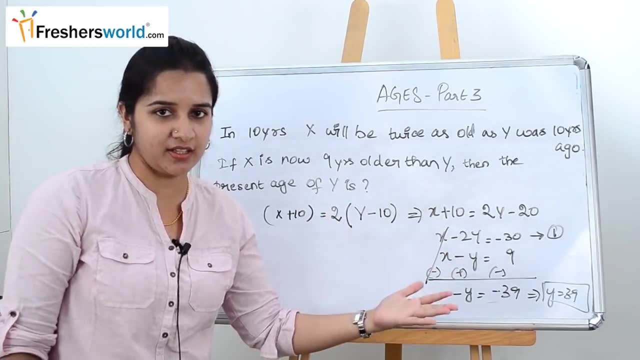 So what are they asking? What is the present age of y? So the present age of y is nothing but 39.. Similarly, in this question they can ask: what is the age of y after 10 years, or before 10 years or various other years given? 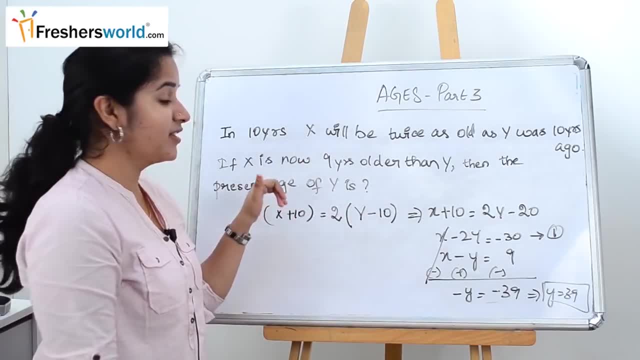 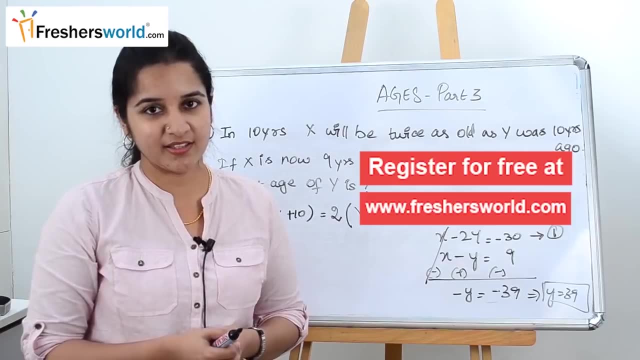 So always make sure you, before selecting the answer, just read the question one more time to finalize your answer. So in the upcoming videos we will be solving much tougher problems in the topic ages. So if you are a person who is looking for a job, kindly register in our freshersworldcom.